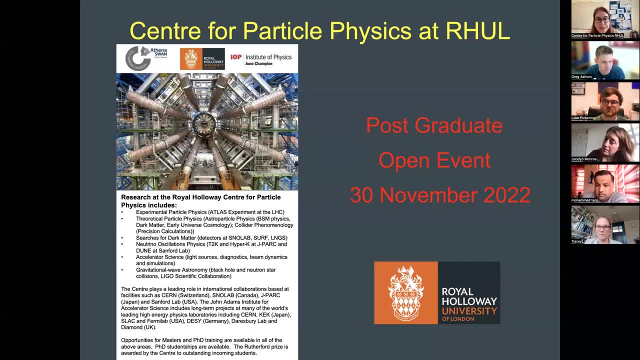 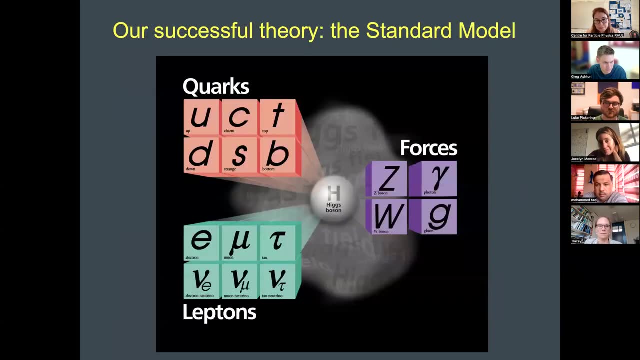 PhD students, in case you want to ask sort of questions that our PhD students will be happy to answer. So hopefully this is all good with you and we'll have a good time this afternoon. So let me get started with our center. So, particle physics, so the kind of research that we do, is where we look. 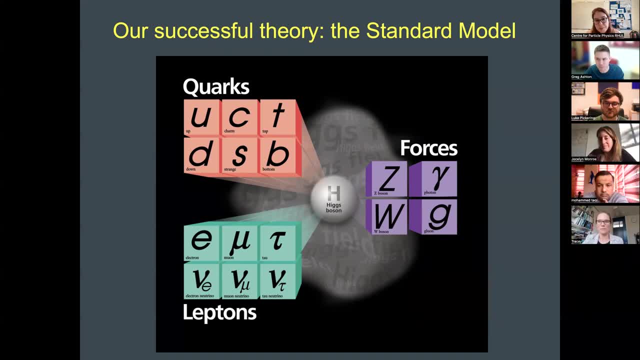 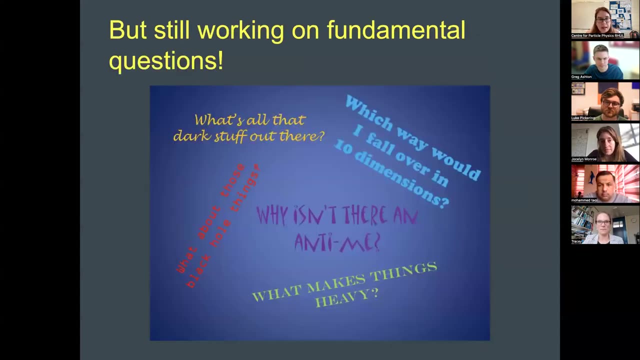 at fundamental constituents of matter, So the fundamental particle, also their interactions, and we have a very successful theory that link together all these different ingredients, which we call the standard models. But actually there's quite a lot of things that we're still asking ourselves about. 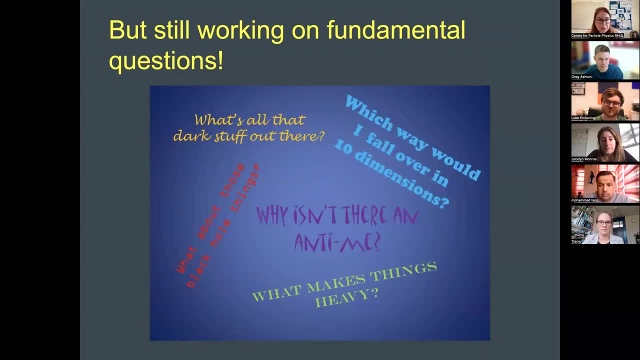 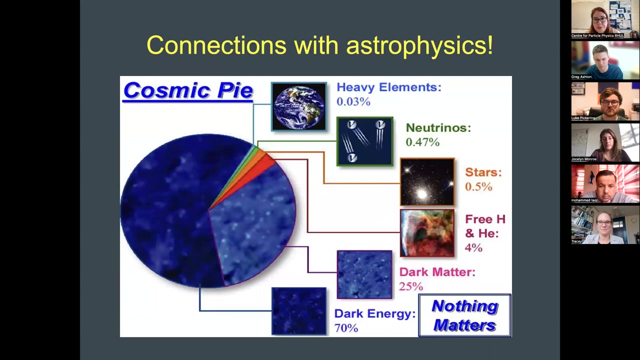 like, for example, what's dark matter? Are there such thing as mini black holes? What gives mass to particles and sort of very sort of precise way? maybe there are extra dimensions out there? So all sort of questions like that that we're still trying to answer, And all of this, what is quite 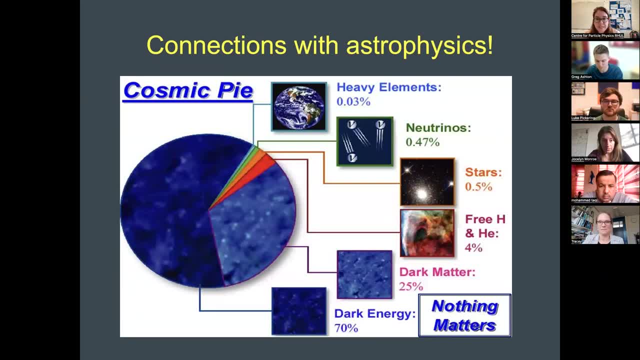 nice is that there's quite nice connections to astrophysics. So normal constituents of matter are actually quite a small part of the energy density of the universe, And so dark matter fits in that. and also we can get information from particle physics, from more astrophysical sort of observation. 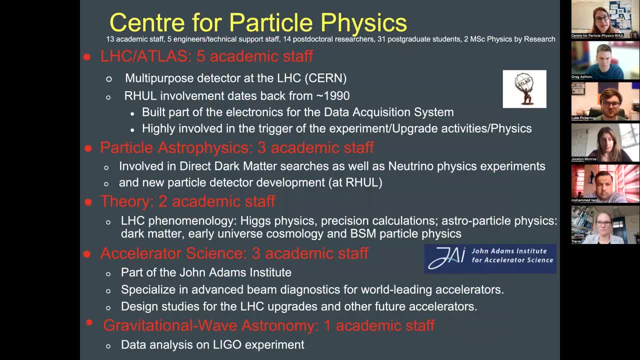 as well. So our, our center has about 13 or so academic staff. we have some engineer and technical support staff, We have postdoctoral researchers and we have quite a large group of postgraduate students And we also have typically some masters students. So you can see here the list of the different research group that 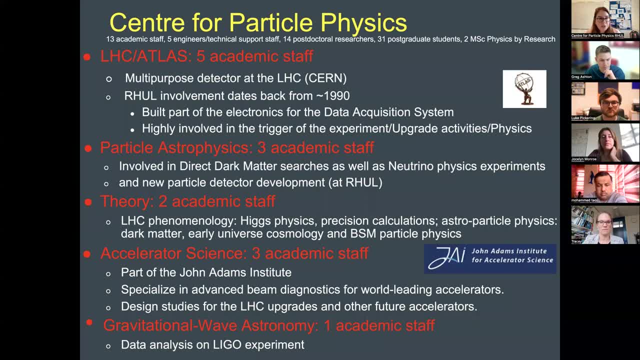 we have. So we have a group working on the Atlas detector, which operates at the Large Hadron Collider. We also have particle astrophysics, which includes direct dark matter searches and also neutrino experiments. We also have theorists that work in. 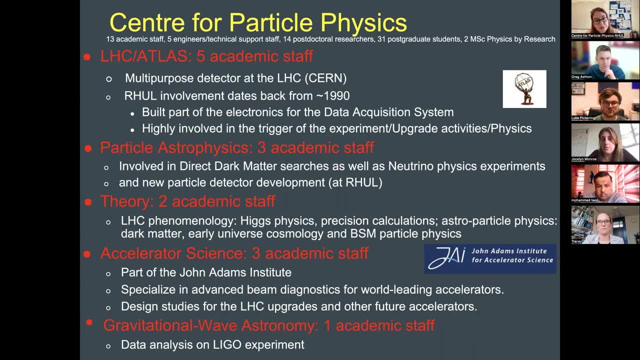 all these different areas connected with our experimental activities. We also have accelerator physics research, part of the John Adam Institute, which you will hear about, And finally, we also have some involvement in gravitational wave astronomy, which you will hear about as well. 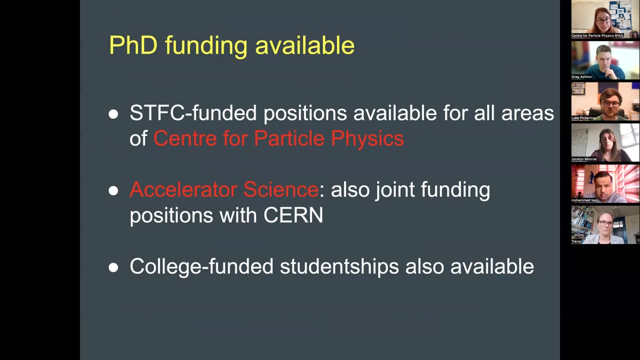 So our position tend to be STFC funded position. So STFC is the name of our UK government research funding body, And so this is available in all areas of the Centre for Particle Physics. Sometimes we also have joint fundings with different labs, like for example with CERN or other bodies, So you can ask. 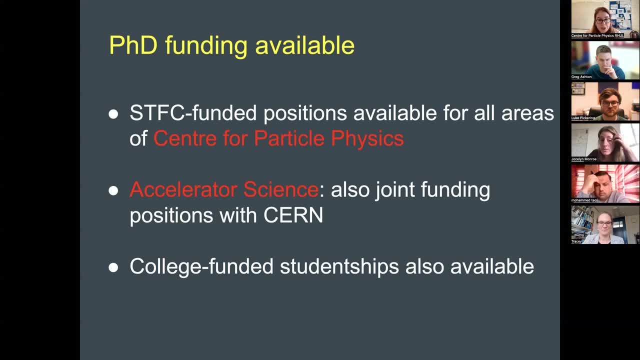 about that as well, And then at college level we also have some amount of studentship available, And so I'll be able to- I'll be happy to answer any question about funding. This funding tends to be open, in principle, to international applicants as well, But the funds there are a bit more limited. 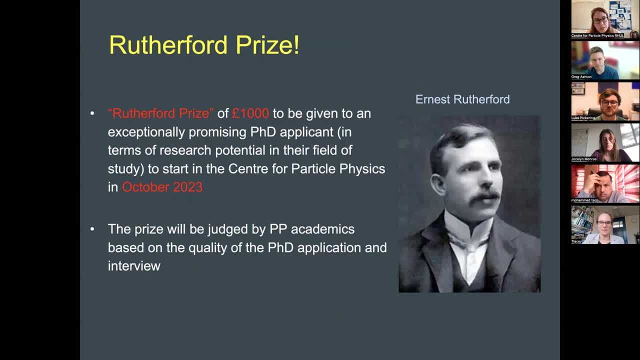 than students from the UK. We have something called the Rutherford Prize, So this is a prize of £1,000 to be given to an exceptionally promising PhD applicant in terms of their research potential in their field of study, And so this would be for somebody that's planning to start in October 2023. And this prize is judged. 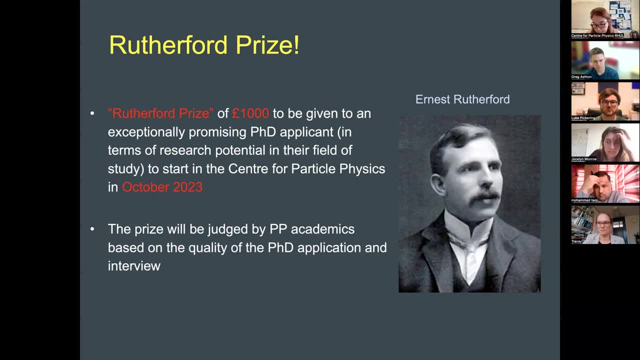 by the academics in terms of their quality of application and the interview as well. Good, So I will now pass on to the different research groups so that they can give you a very short introduction to their research and the different academics working in that area. So first I'll 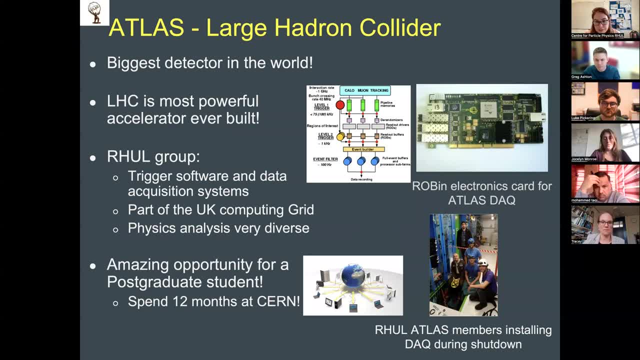 give the floor to Dr Berry, who will talk about ATLAS. So, hi, I'm one of the about four or five lecturers on academics working on the ATLAS detector. So the Large Hadron Collider, as you know, is very large, the largest hadron. 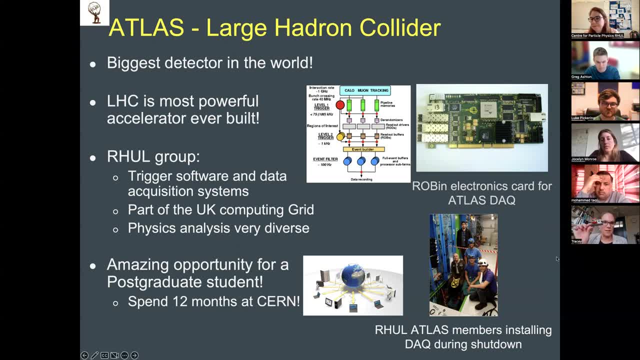 collider in the world And ATLAS is the largest detector in the world And we have a little mini-scale figure that you can do with the outreach with our group as well. So, as you know, the LHC is very powerful. It's 27 kilometres per string and it's now accelerating protons. 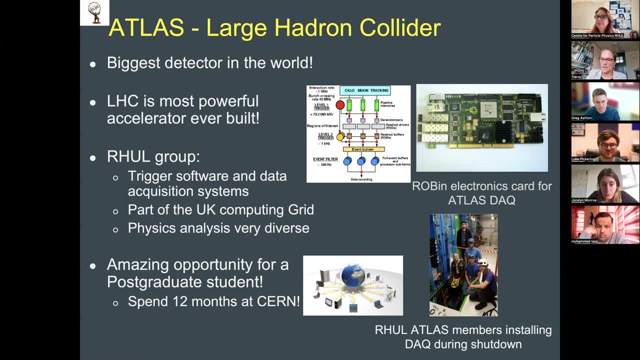 and protons to collide at 13.6 TV, which is the highest energy ever in the world. So now it's a really good time to start a PhD on ATLAS, because we're actually in data-taking phase and will be for the next few years. The Royal Holloway group in particular specialises 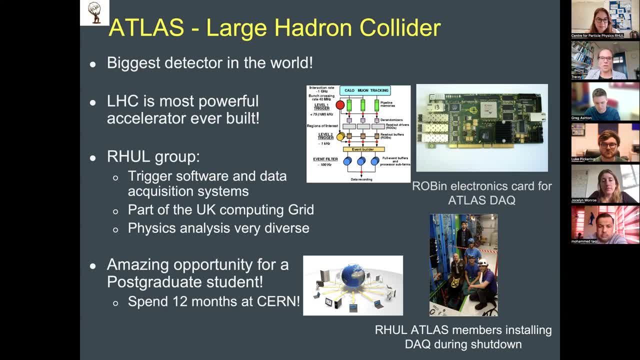 in the trigger software and data acquisition systems. We're also part of the UK computing grid and we have various different physics analyses, as I'll go through each of the topics in a minute. So it's an amazing opportunity for a PhD postgraduate student to work here. 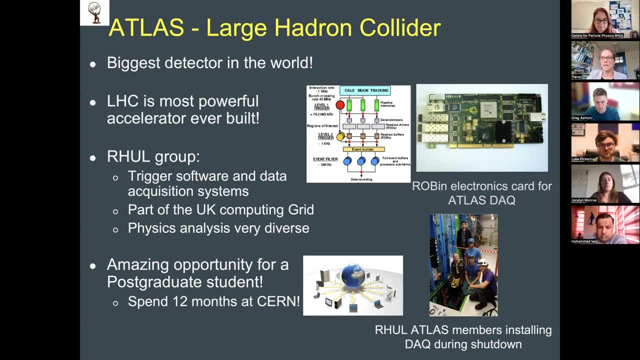 at Royal Holloway for some of the years, but also to spend 12 months, typically in their second year, And here's a picture of some of our students in the bottom and staff members actually installing things in the ATLAS detectors. So on the next page, I'm not in control. Yeah, thank you. 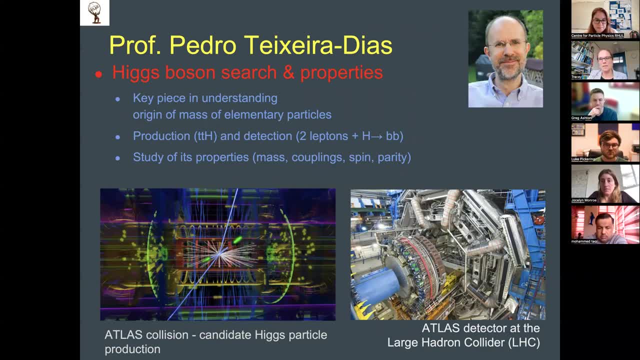 Yeah, So to work through the projects in particular. so Professor Texi Adiris. it's a specialist who works on the Higgs searches and was involved in the Higgs discovery back in 2012.. And now he's working on- and his group are working on- understanding the properties of the Higgs. 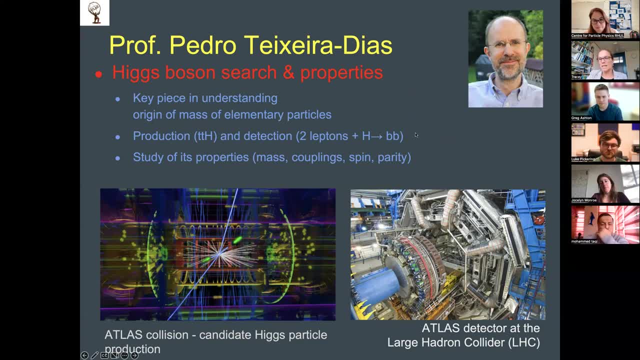 In particular, he's specialising in the TT Higgs production and its decay to two leptons, and the Higgs decay to two b b b, b b b b And they're using this to study the properties of the Higgs. Now we've discovered it to, for example, to find its mass couplings. 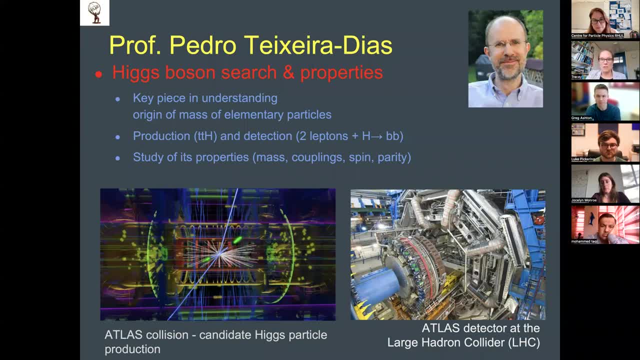 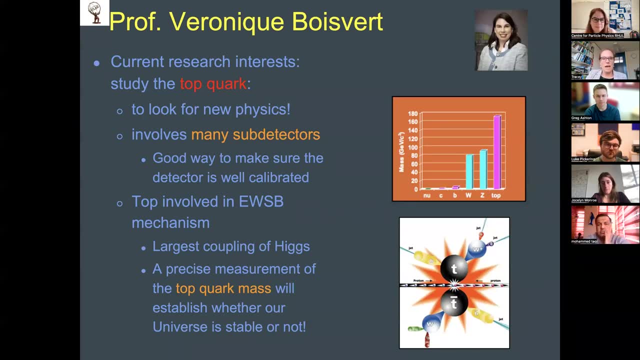 its spin and its parity. So he's an expert in that area and has a group on this. Also we have Professor Borellet, who's just done the introduction here. She leads the group and she's a specialist in looking for top quark. So the top is the heaviest quark much. 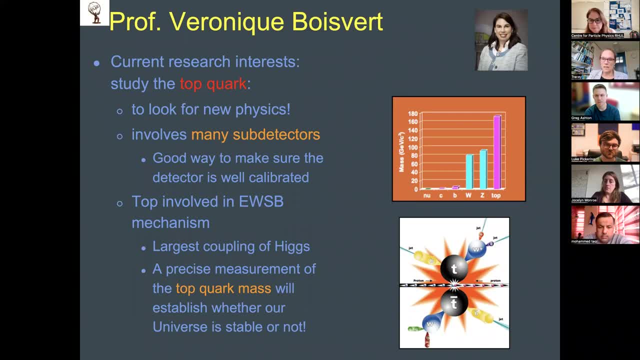 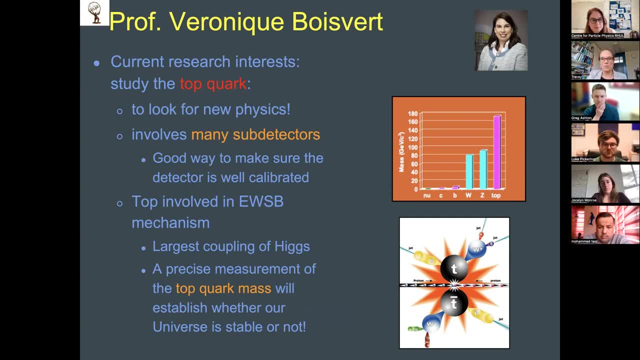 And it's very interesting to look for because it involves decays, involve all the different sub detectors in the Atlas detector, So it's really good to calibrate the detector at the start of a run and also then to do a very good detailed physics searches with that. 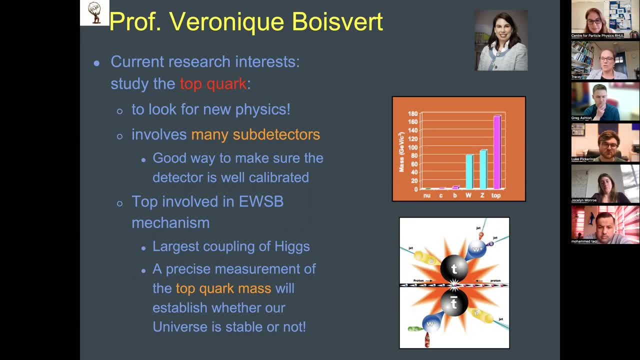 As well as studying the properties of top quark itself, you can use the top quark to look for new physics and look for beyond the sun model physics and various decays or properties related to that and how it decays, And you can actually use it to study precise measurements. 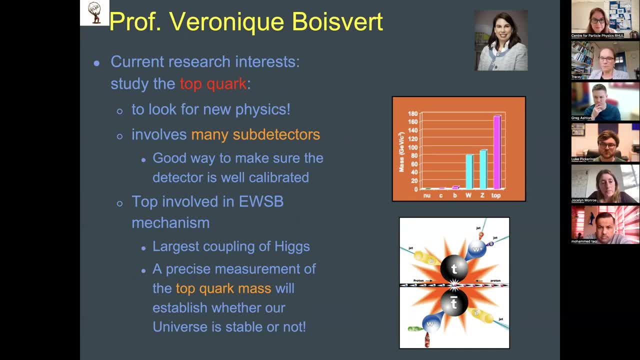 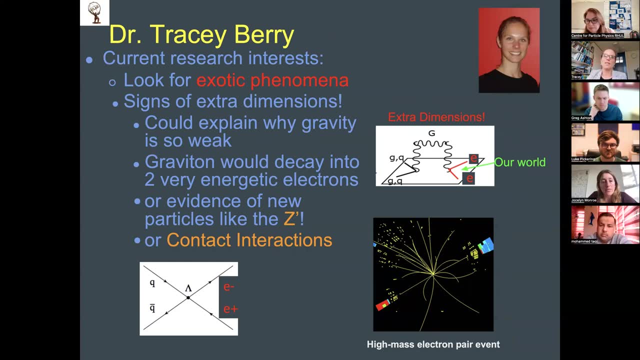 of it to enable to discover whether the universe is stable or not. So it's very exciting. The next one is me, So I search for exotic things, so things that are beyond the standard model as you know it. So I'm looking for things, for example, X dimensions. 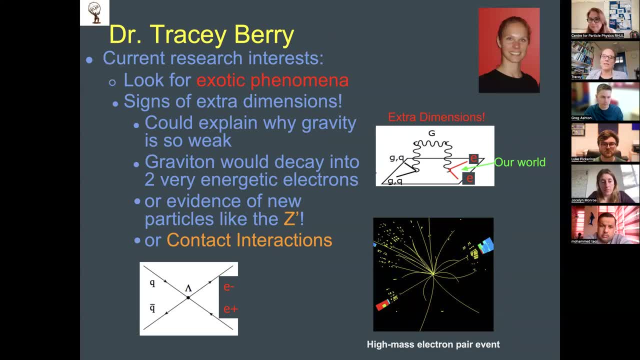 And this could explain why gravity is so weak. And lots of things I search for decay in such a way that they result in two high mass electrons. So, for example, a graviton, it could decay. It would go into X dimensions, but it would decay into our standard model particles. 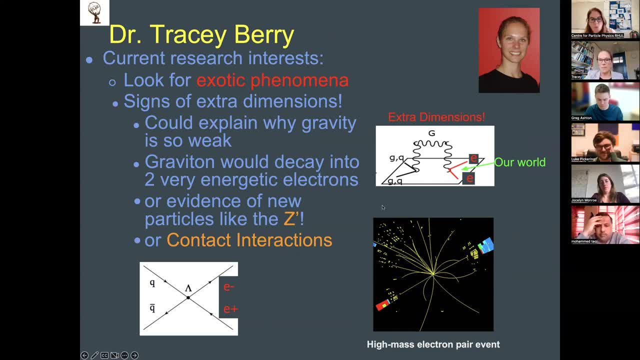 So we would observe a deviation to our standard model expectation. So I look for two high mass electrons, either for resonances or a broader excess at generally high invariant mass. And I'm also looking at low invariant mass because you could find such things as dark photons. 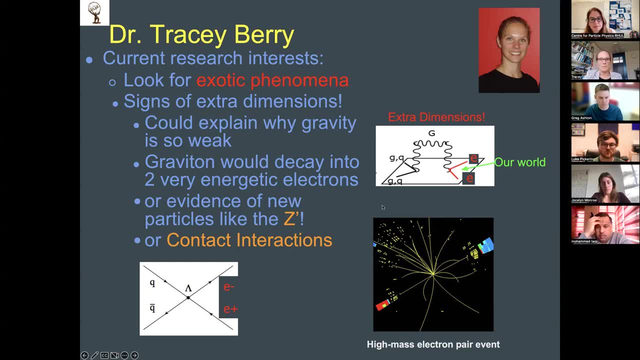 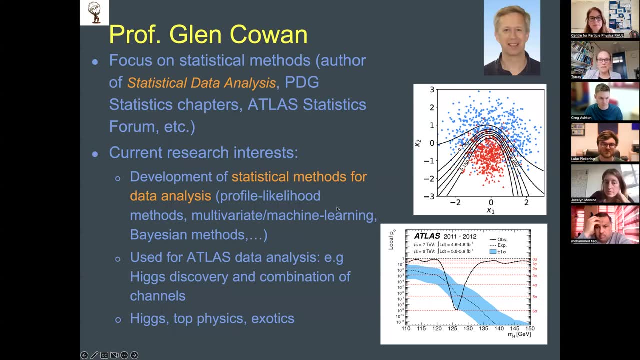 Also new resonances, Z primes or content interactions. And then, finally, but definitely not least, is Professor Glenn Cowan. He's an expert on statistical methods and he's actually author of the Statistical Data Analysis book and the PDG. He writes statistics, sorry. Statistical Data Analysis book. 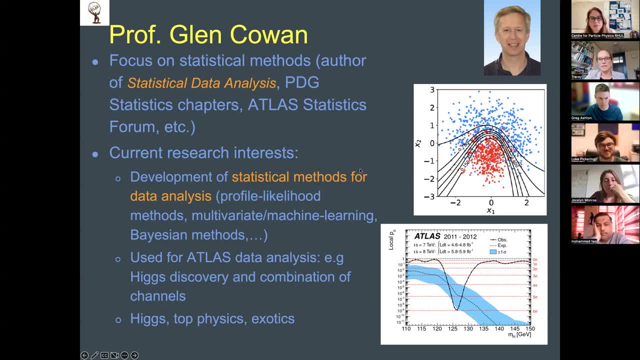 He writes statistics, He has chapters on the PDG book and he's also the statistics forum expert. So he does many different. he's involved in many different searches, particularly when he's looking at some Higgs and TOPS searches, But he uses works on the statistical methods for lots of data analysis topics. 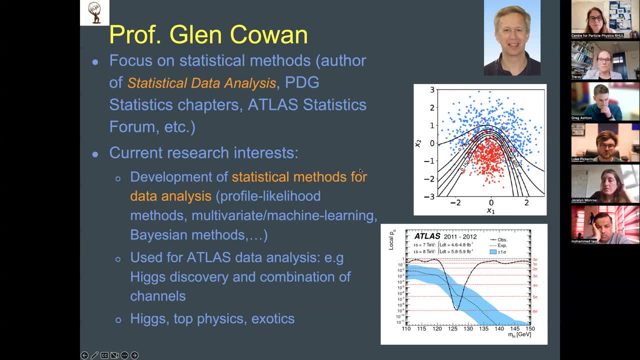 And so it's implemented in many different analyses. He's specialised in profile likelihood, machine learning, multivariate techniques And he's basically generally involved in lots of combinations. So he's involved in the Higgs combination paper. So that's a very good book. 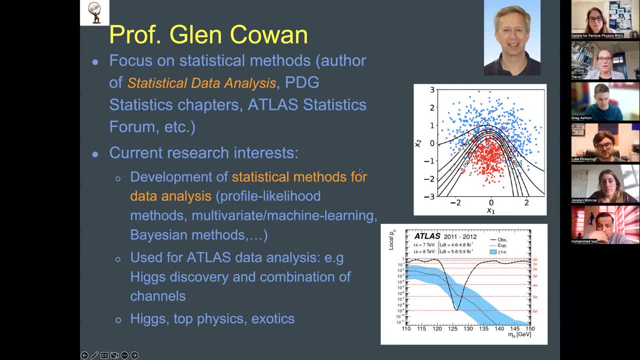 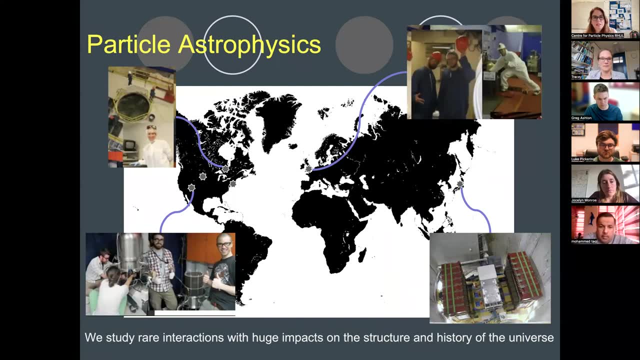 It's a very particular, a good topic and covers many different searches. So that's the highlight for the Atlas group And you see we've got a wide group and lots of different interests. Okay, Thank you very much. So now we can move to the particle astrophysics, and I think Professor Munro will kick off there. 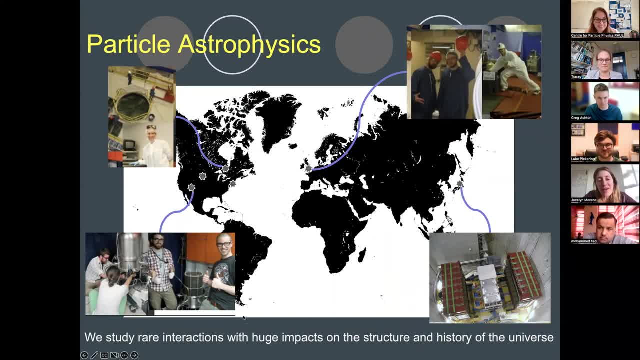 Hi everybody. I'm Jocelyn Munro, So my research is in dark matter and neutrino physics. So we do particle astrophysics experiments in our research group around the world. So you can see some pictures of our students in various facilities. 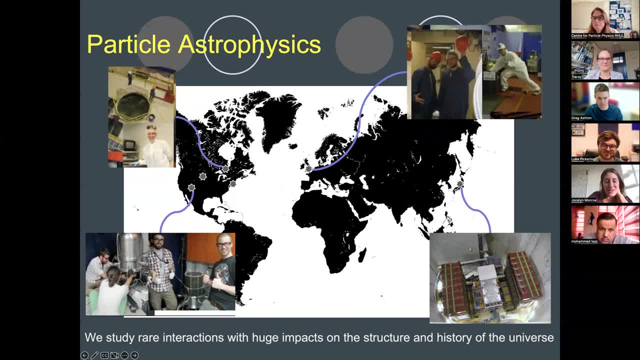 So we do experiments that are at Snow Lab in Canada. We've done experiments at the WIP facility in the US. We do experiments in Japan at J-Park. We do experiments- I've missed one- in the US- actually at SURF in South Dakota. 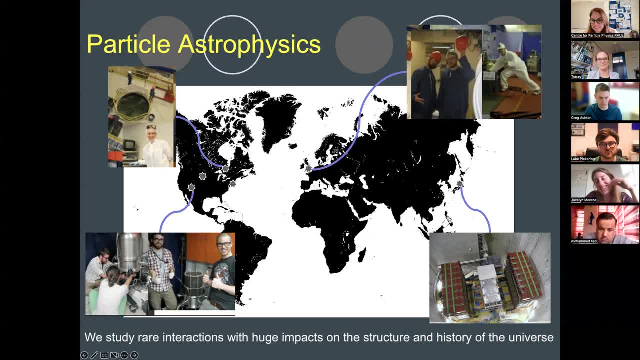 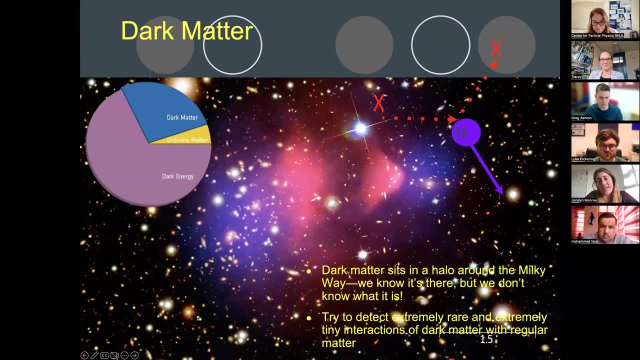 And I'm working on building an experiment now that's underground in Italy, in the Gran Sasso Mountains, And so if you like to travel, we're the group for you And we have a strong focus On detector development in this group, And so we kind of do a combination of data analysis and detector development. 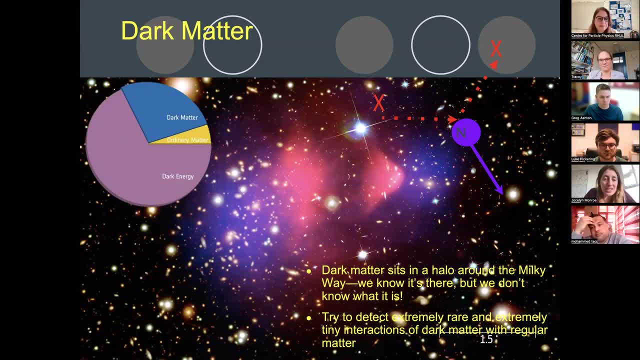 So the problem that we're going after is to understand the nature of dark matter, which we think makes up more than five times as much of the energy density of the universe as all the particles we know about in the standard model. So in this pie chart that you see in the top left here, standard model particles are this kind of yellow slice. 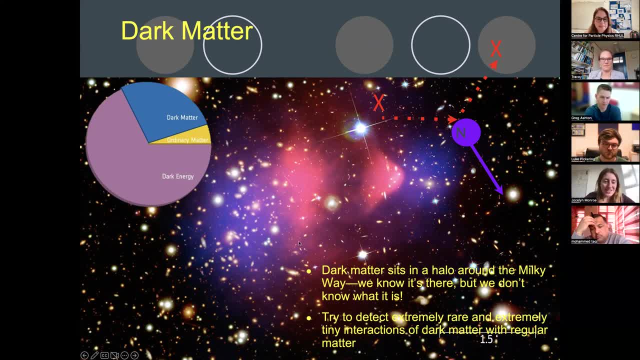 Dark matter is the blue chunk and the rest we understand even less about. That's dark energy, And so we think that dark matter sits in a halo around the Milky Way. We know it's there, but we can't see it interacting with photons through our telescopes. 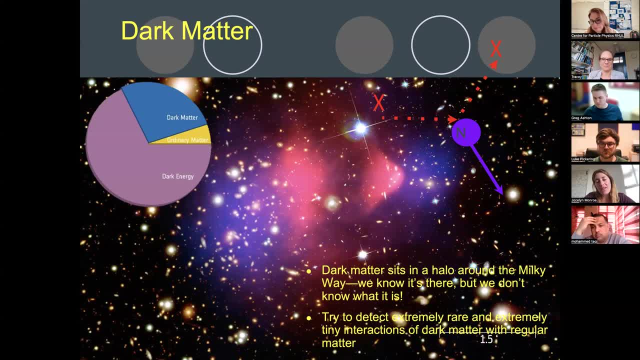 And so we build experiments that look for some evidence that a dark matter particle scatters off some atom in an ultra sensitive terrestrial detector And we try to measure what that recoiling atom does. So there's kind of a cartoon of this process which has shown that the dark matter particle flying in and out in red. 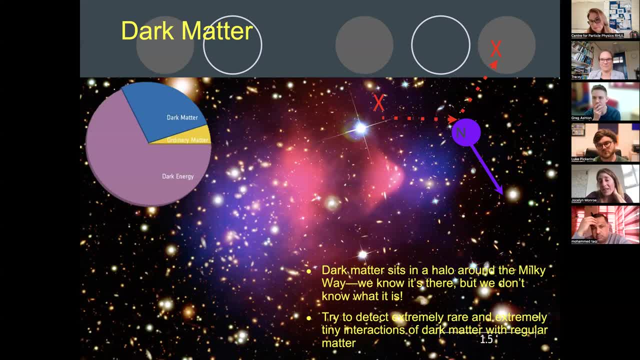 We don't see that, but what we can hope to detect is what the particle it hits does, And so this purple arrow is kind of schematically illustrating a recoiling nucleus through a detector. So this process is extremely rare and it deposits an extremely tiny amount of energy in the detector. 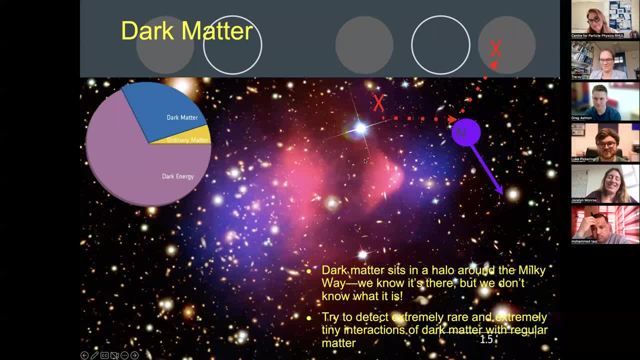 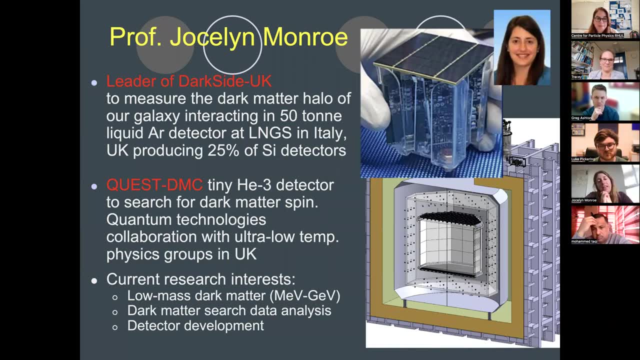 And so these experiments are extremely technologically ambitious and hard and it's a great project for a student. So if you go to the next page, So I work on the DarkSide 20K experiment. There's a schematic of the detector below here. 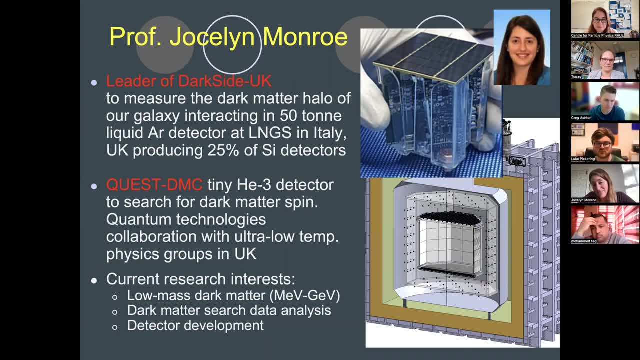 This object that you see in this big gray square is eight meters on a side, So it's quite a large instrument, And I lead the UK groups and we are building a quarter of the ultra sensitive photon detectors. which instrument this detector? And so one of them is shown in this picture in the top right. 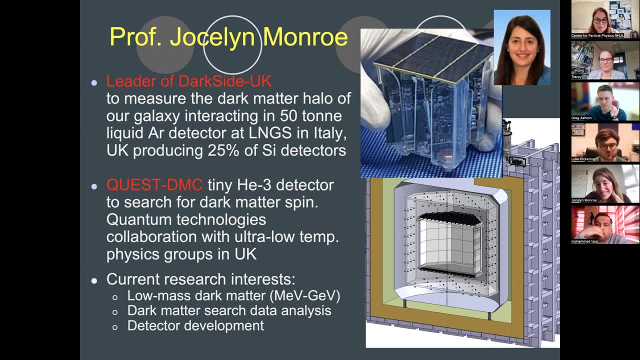 You can see, it's the size of your hand. We're building seven square meters of those here in the UK And that's a quarter of the total And those will help instrument the largest dark matter detector ever constructed. It will have a 50 ton argon TPC at its heart. 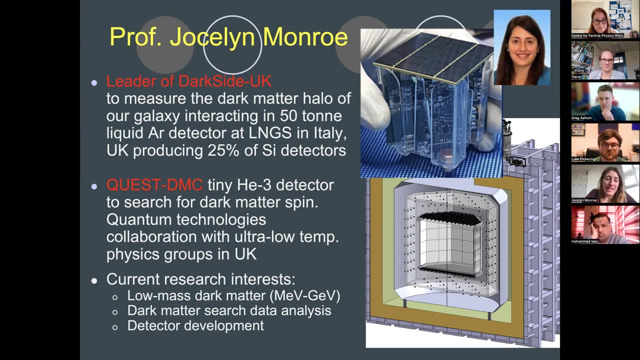 It's located in the laboratory. Oh, that's Melody Gran Sasso in Italy, and it's under construction now. So it's a great time for students to get involved and be part of the kind of commissioning of this detector and turn on and first science towards the end of your PhD. 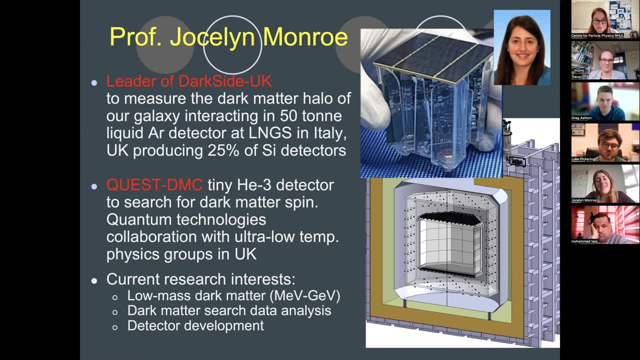 So we're definitely looking for students there. I also collaborate on an experiment at the other end of the scale, which is a tiny one cubic centimeter experiment filled with superfluid helium three. We have to operate at 150 micro Kelvin in order to get it to a superfluid state and we're looking there for dark matter. 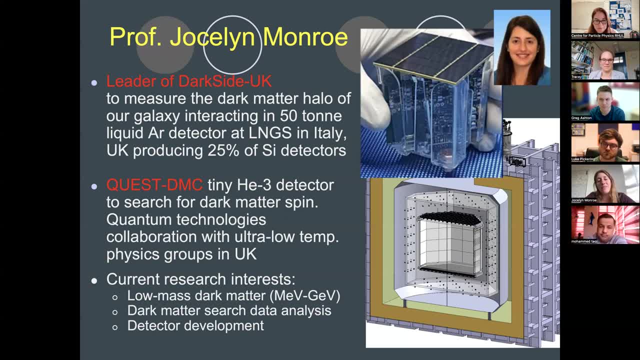 So we're going to try to get the particles to interact in this tiny detector and actually interact with the spin of the helium three atom, And we instrument this object with quantum technologies and this is a collaboration between our dark matter group and the ultra low temperature group. 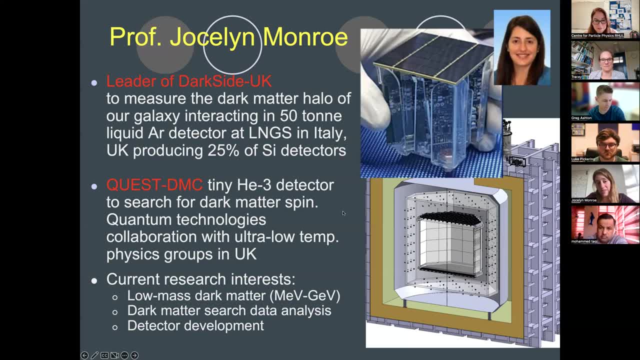 I'm here and also in Lancaster, and we also have a PhD student opening on this project this year, And so the thing that kind of knits these together is we're interested in both of these projects and looking at low mass dark matter. 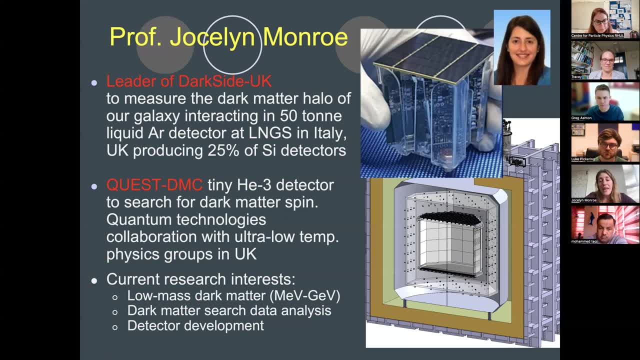 We're interested in developing new dark matter analysis tools And, as I kind of already mentioned, our focus in terms of the instrumentation is on detector development of novel techniques to look for these instruments. So in our group we have dark matter and neutrino physics together because 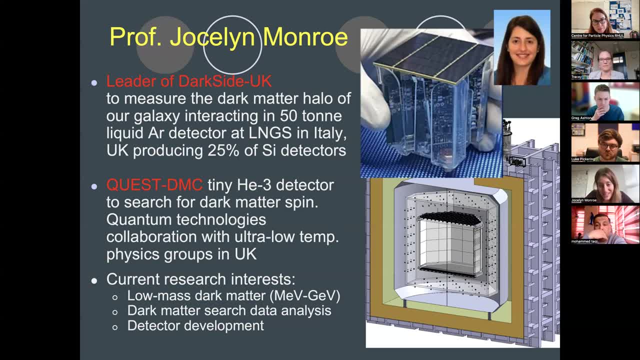 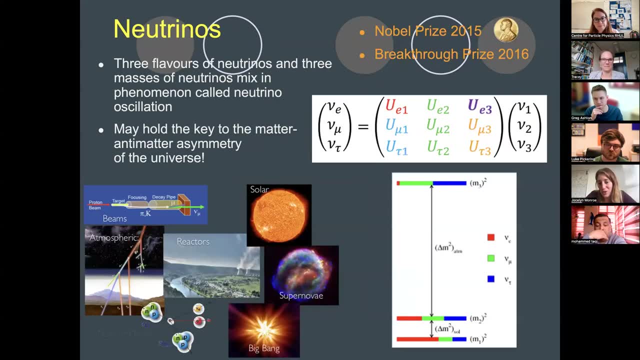 a lot of the challenges are the same. Neutrinos are also particles which are very hard to see, interact rarely and require some of the same detector technology. So I'm going to turn over next to my colleague Luke, who's going to talk about what the other part of our research group. 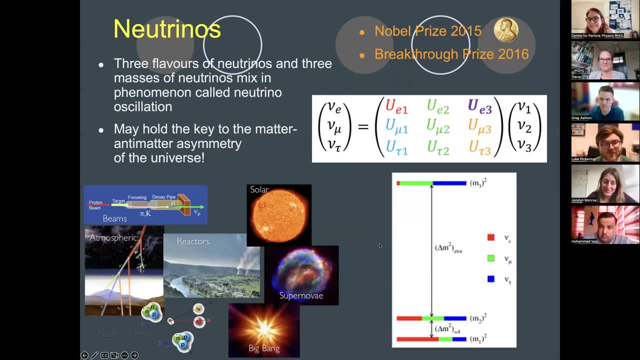 does on neutrino physics? Hi, yes, I'm Luke. So yeah, neutrinos. you know we have these sort of shown in the matrix here. We know in the standard model there are three flavors of neutrinos and we know that we can create a beam of neutrinos, which is kind of exciting. 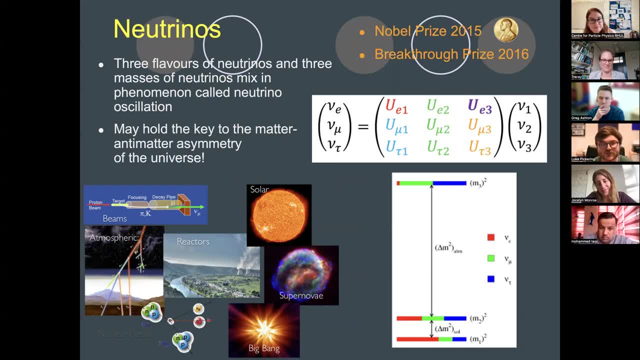 There are sort of millions and billions of neutrinos going through you every second, producing the sun and, if you're standing in the right place, producing our beams, But they interact so weakly that you need these huge detectors to be able to see them. 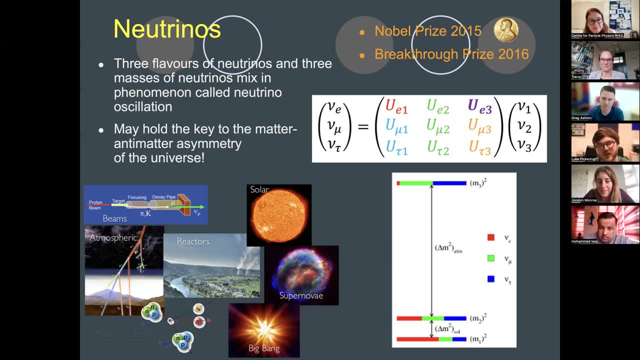 And the property that we're really trying to sort of work out about neutrinos is this property called oscillation, where we can produce a beam of neutrinos in this muon flavor and then detect them hundreds of kilometers later and find that they have. 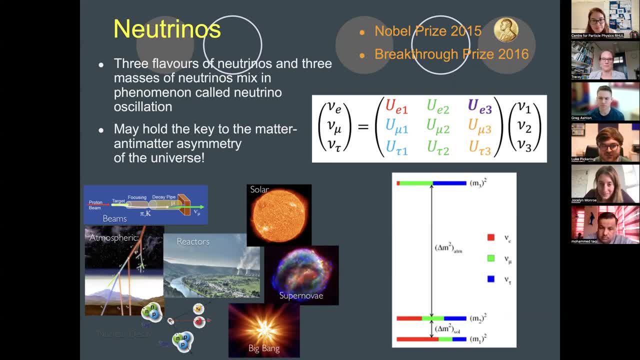 changed into electron and tau flavor, And the thing that's really exciting about this is that it's sort of a quantum mechanical process that happens over hundreds of kilometers, rather than you know the much smaller scales we're used to. As Josh has already mentioned, the group is kind. 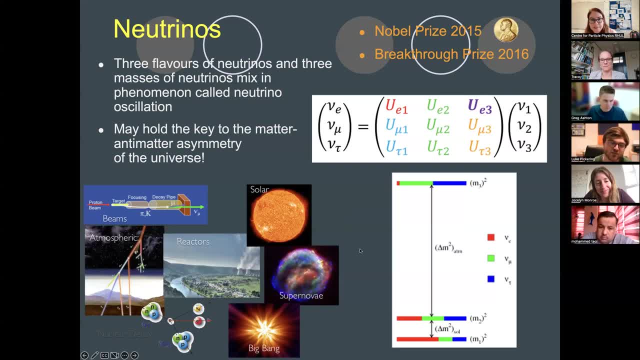 of involved in this. So we're going to talk a little bit about that. So we're going to talk about this. So we're going to talk about this, So we're going to talk about this. So we're going to sort of both detector development but also analysis. This is split between an experiment. 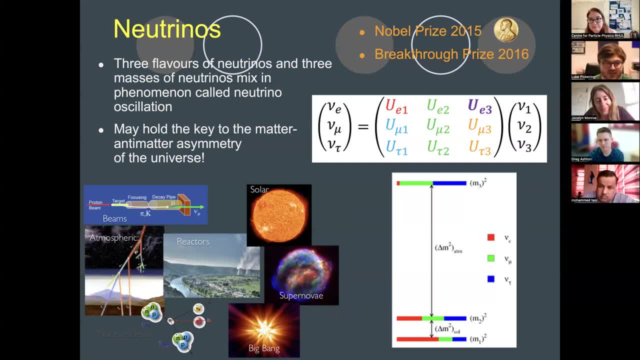 in Japan called TTK, which we're running, and has been running for 10 years, where we're mainly analysis focused, trying to do precision measurements of this neutrino oscillation process And, at the same time, looking forward to the next generation, which is June, where we're 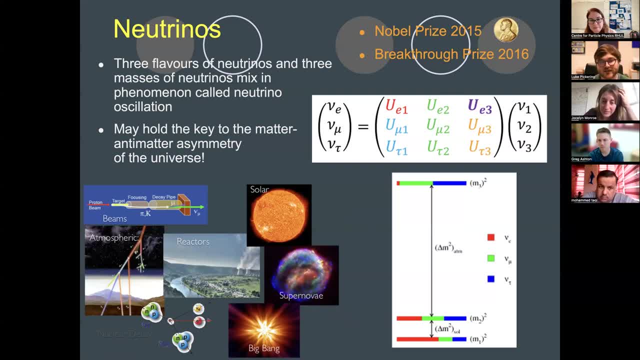 building an experiment that's expected to start taking data in the 2030s, early 2030s, just outside Fermilab, just outside Chicago, sorry, and a national lab in the US called Fermilab. While we know this process of oscillation happens, there's, there's still lots of sort of 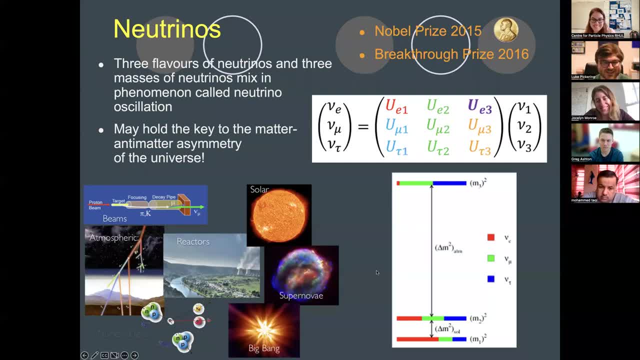 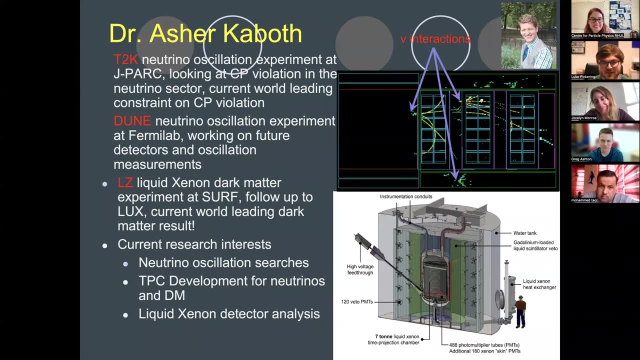 precision measurements that we're doing, Sorry, And so we can move on to the next slide. So first of all, Dr Kabath, sort of our colleague and the person tying this neutrino dark matter group together, because he's the one who's really split in half, he's led the way historically on doing 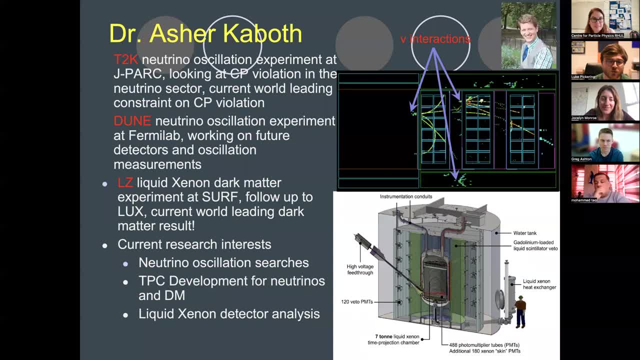 these oscillation analyses on TTK, Also working on the future experiment June, where he's working on developing a new sort of concept of detector for this near site. So remember I said that these beams we create are left to travel for hundreds of kilometers. 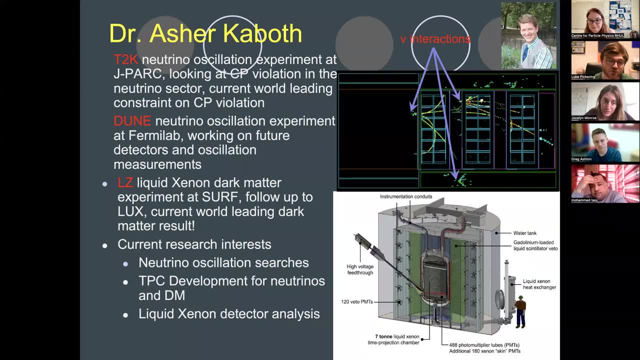 we sample them near, where we create them, and then far away, a so called fire detector. we're mainly focused on playing with the near detector in June, And then Asher also works on LZ, which is a liquid xenon dark matter experiment at SURF, which is a Sanford Underground Research. 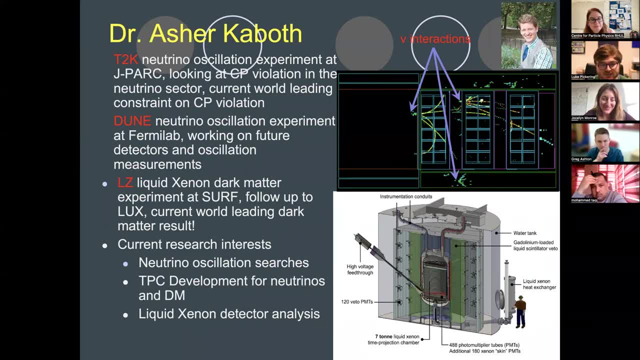 Facility which, coincidentally, is also where the June fire detector will end up. So there's lots of interplay between these two fields, as we've heard. So on to the next slide. I'll briefly introduce me. So yeah, on the TTK. 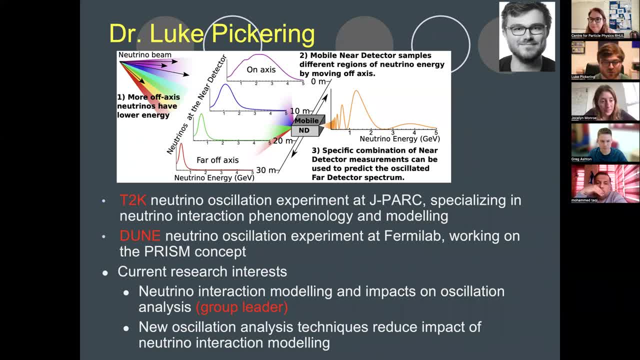 side. I'm mainly interested in trying to work out how well we understand, or don't understand, how neutrinos interact with matter. We know they interact very rarely, But depending on exactly how they interact, we can introduce subtle biases into the measurements that we make. So we've got 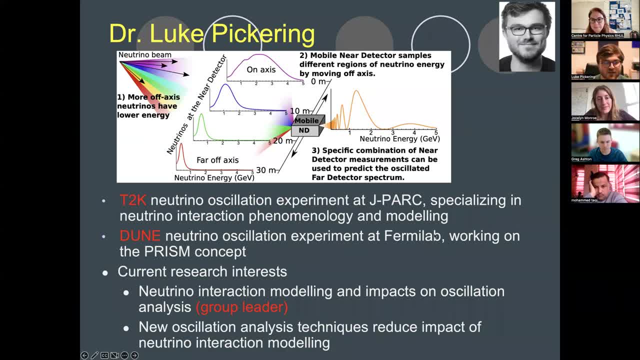 to you know model how they interact with matter. So we've got to you know model how they interact and also uncertainties around that. So that's what I play with on TTK On June. I'm trying to sort of make a near detector concept that sidesteps that problem that I mentioned, that we 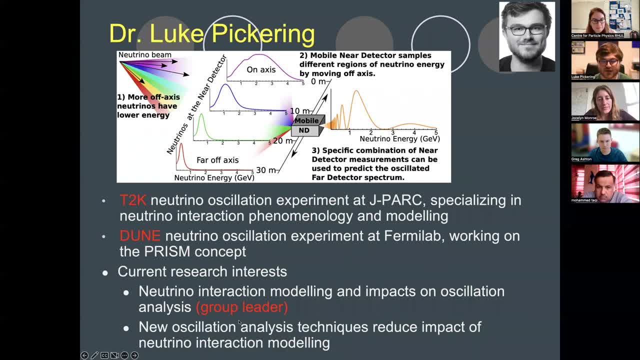 have to deal with on TTK And the kind of central part of that is that we're able to move this sort of 100 plus ton detector And by moving it in and out of the new beam of neutrinos we can sidestep. 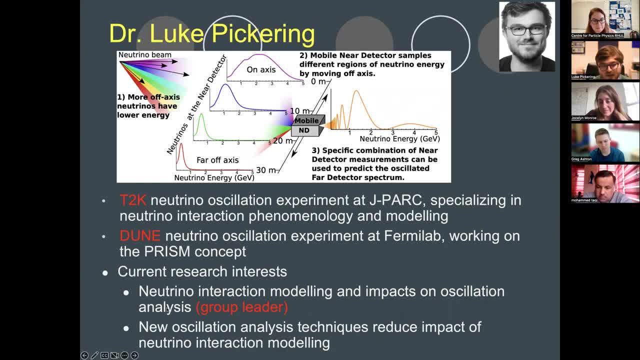 that problem with how neutrinos interact. So yeah, those are my interests And I think you know I'm sort of ramble flowing enough, So I'll hand on to the next person. Great, Thank you very much. Very interesting, And so next we have Dr Kaur who's going to. 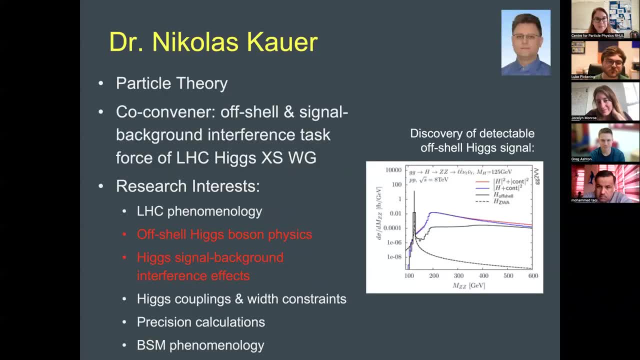 tell us a little bit about our theory activities. Hello, can you hear me? Yes, Great, Thank you. So I'll just introduce you to the theory activities in the particle physics group. And so there are two different research directions. One is focused on 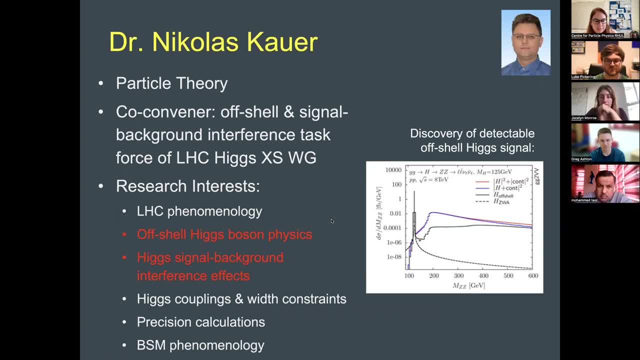 the collider phenomenology and more of a focus on precision calculations and also new physics studies, And my personal research interest has been an option- Higgs physics- which is complementary to the standard on peak resonance studies and led to some interesting observations. 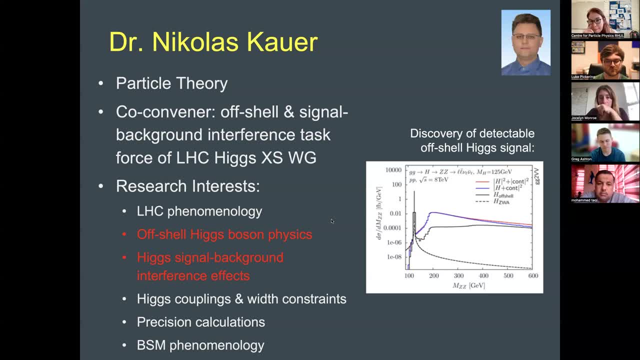 displayed in the graph. So the regular peak is here Shown in the graph, and then the offshore region starts at around 200 GV and contributes surprisingly, about 10% to the actual Higgs signal and can be used as a complementary source for. 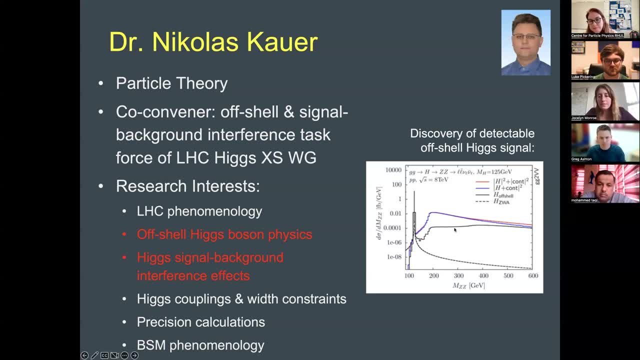 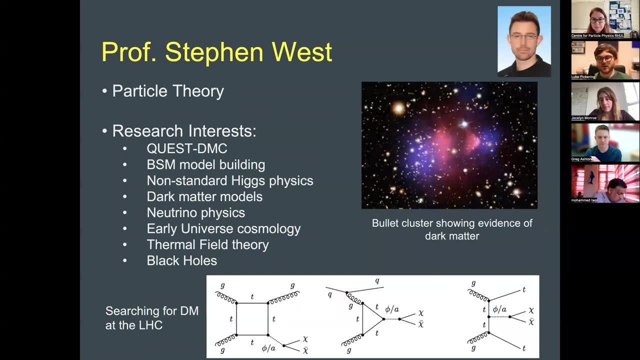 Higgs property studies. Next slide, please. And my colleague, Stephen West is interested in dark matter physics and also in cosmological questions. early universe thermal freezeout was a main topic he worked on. also interested in black hole studies And there's a picture of the bullet cluster that 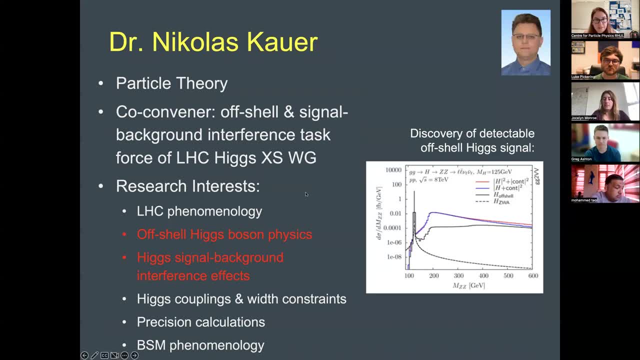 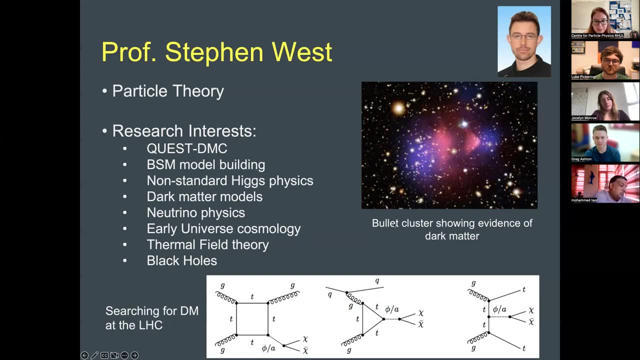 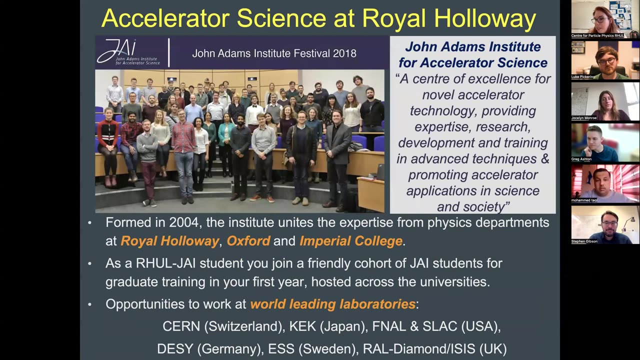 shows evidence of dark matter. So we have two complementary directions in the theory group here. Great, thank you very much. Next is going to be our accelerator physics, which is going to be talked about by Professor Gibson, who's also the head of the physics department here at Royal Holloway. 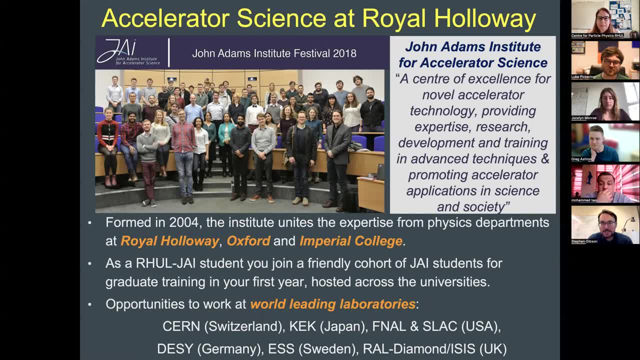 Hi, hello everyone. So I'd like to talk about the John Adams Institute for Accelerator Science. So this is a grouping of universities- Royal Holloway, Oxford and Imperial College- And we basically build and develop future accelerators. So if you were to join us here at Royal Holloway, we're going to be doing this in the next few days. 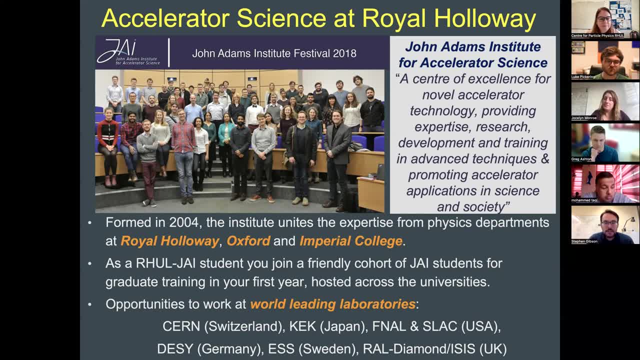 here at Royal Holloway. you'd be a part of this wider team as well as having local supervision here, and we typically meet each year and connect with each other. but in particular for the JAI students, you have graduate training in your first year. there's a series of lectures held mainly at 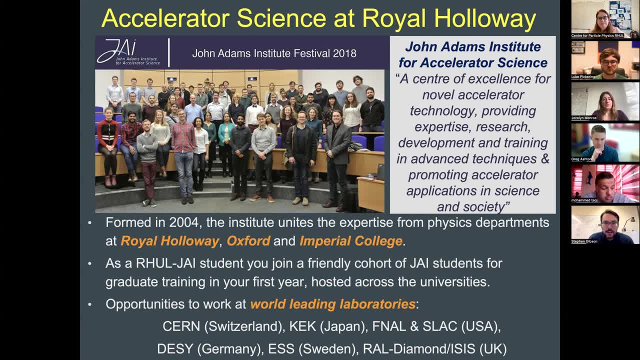 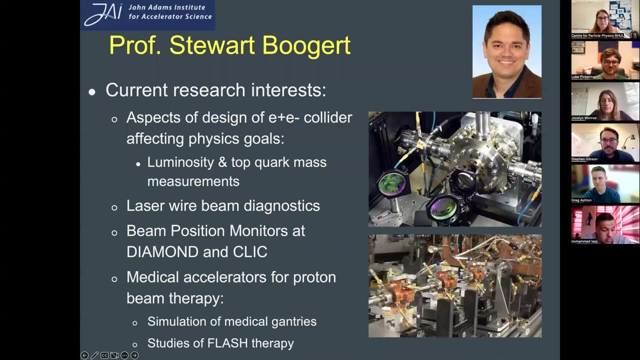 Oxford University that you would go and attend, and there's also opportunities to work in world-class laboratories around the world. so SAAD KAK in Japan and others. Perhaps moving to the next slide, I can just introduce to you some of our group members. so we have Professor Stuart Buget. 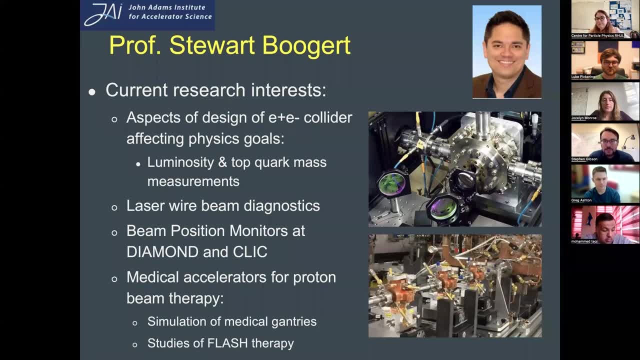 who is a former head of department and head of school here at Royal Holloway and he is active in a number of areas related to beam instrumentation and in particular also simulation of particle accelerators. so thinking also about applying the way that we track particles through complex lattices of magnets. we simulate that, but we also 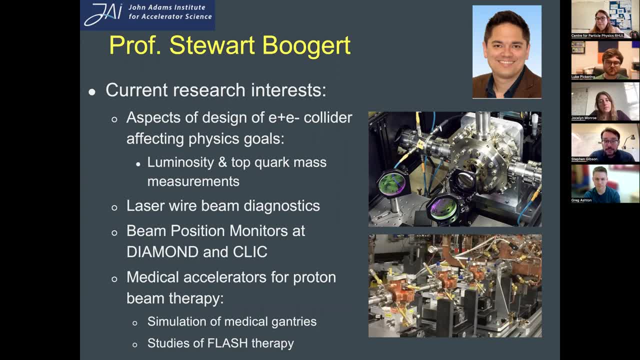 apply those simulations to important applications, for example in medical proton beam therapy, studies of medical gantries. the one hot topic that's come up recently is flash therapy, so some of these things are in the news recently. for example, CERN are currently just announced they're going to collaborate on a very high electron energy machine. 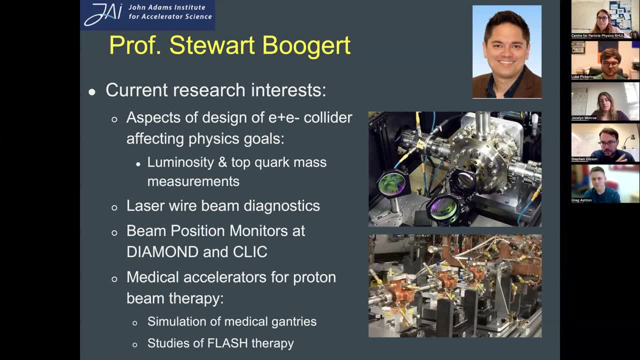 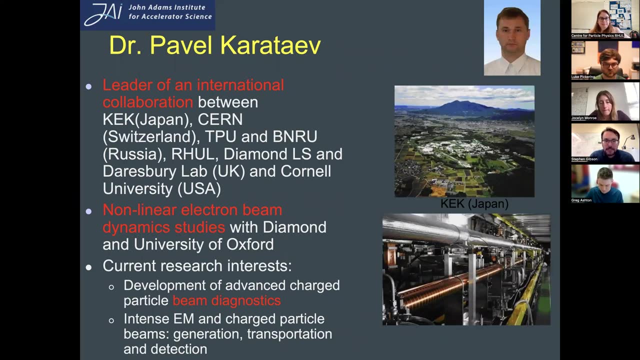 for flash therapy, where you rapidly target a tumor and that, but in such a way that it keeps the healthy tissue intact. Okay, moving to the next slide, we have Dr Pavel Karataev, who is also an expert in beam instrumentation, but in particular in using optical methods to diagnose the properties of particle beams. 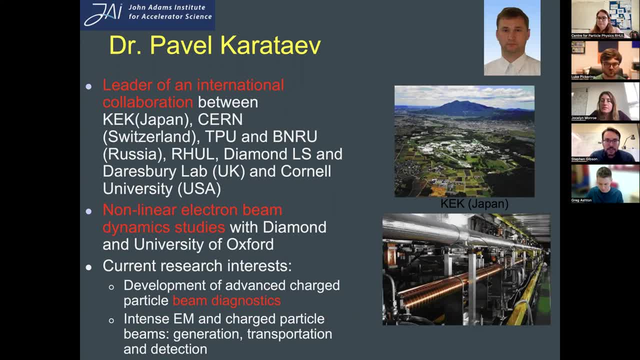 as they traverse and go through the accelerator. so thinking about optical transition, radiation, radiation and other types of novel accelerations. so we work on pyroelectric acceleration. we have a mini accelerator in the labs here at Royal Holloway. and then the next few slides, I think. 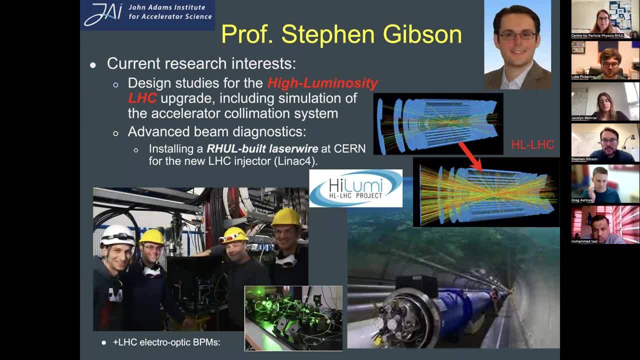 are a little bit of the research that I work on. so this is on the upgrade to the large hadron collider, the so-called high luminosity upgrade, which will increase the number of collisions at the inside atlas, for example, by around an order of magnitude, and we're working on a diagnostic shown on the next slide, which is an 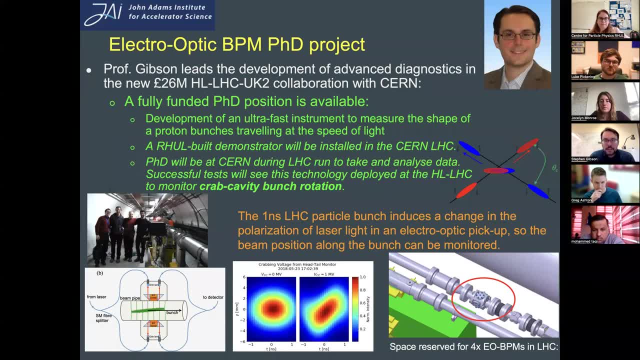 electro-optic beam position monitor which basically measures the rotation of the bunches as as they collide. so in future we're going to what's called crab the bunches, so that when they collide it increases the number of collisions and we're developing a very fast electro-optic pickup. 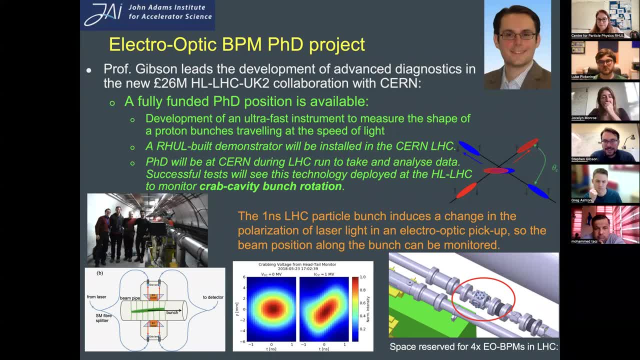 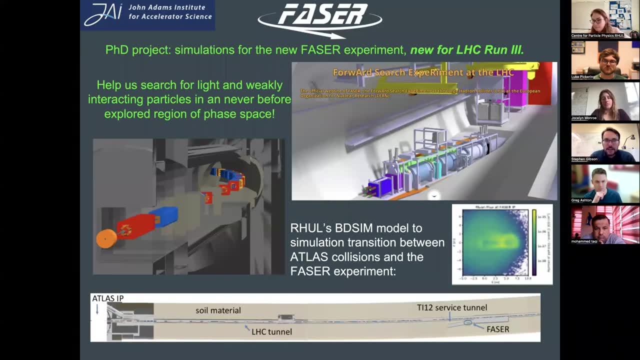 to be able to monitor that, that rotation using clean rooms here at Royal Holloway. And then I think the final slide also just relates to some of the simulations that we do for other experiments at the LHC. so in particular linked with our excellent Justin Monroe's group in 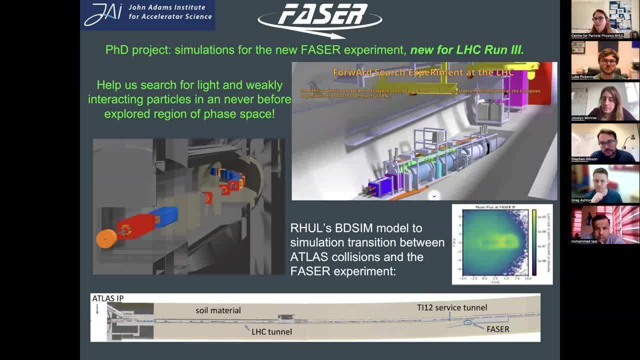 dark matter. we have a study of light dark matter and axions that propagate from atlas to a new experiment called the phaser experiment, which has just started running in run three of the LHC. so this is a simulation in our code called BDSim and you can see how tracks propagate from atlas all the way out to phaser. so 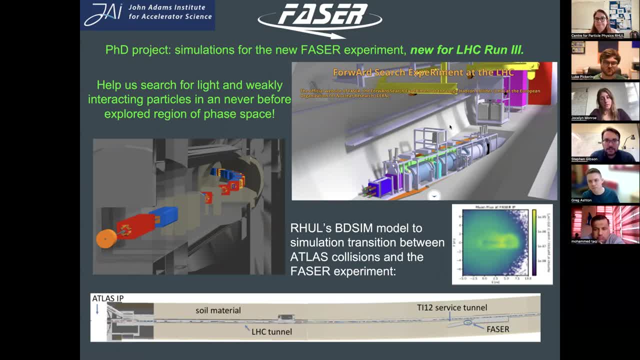 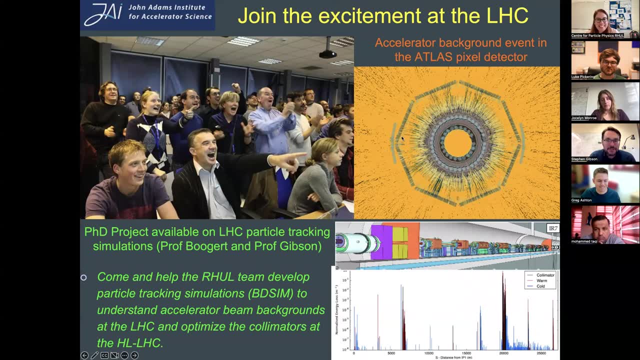 look forward to first data in the coming months at phaser. okay, I think that was the last slide, is that right? yeah, just to join the excitement here. oh, yes, that one. I forgot that. so that's the old slide, but it's just from some of the first startup events at the LHC. 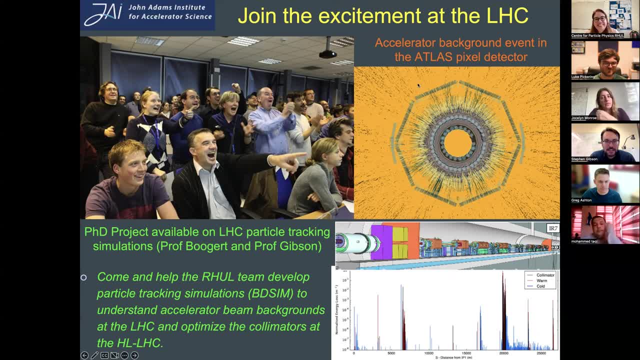 you know that's me. I can do the pose, but, yeah, we work on particle tracking simulations for the LHC as well. so lots of ways in which we can apply the knowledge that we have to develop and investigate accelerators. so, yeah, feel free to chat to me later if you'd like to get some more details on specific projects. great, thank you very much. 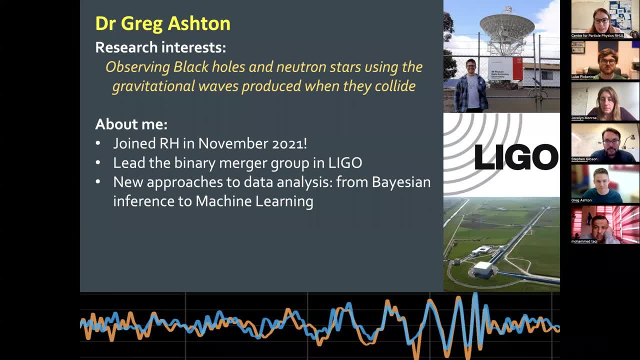 And our last activity is on a gravitational wave and Dr Ashton is going to tell us more about it. Graig Ashton- animator. Hi everyone, my name is Graig Ashton, and so we've heard lots and lots about partmelata and much more about how those llegar. particle tracking project over the last few years has been essentiallyado a roadside Metro ost meant a great or lots of interesting IT-like aspects to do, and so results have been incredible and all working out to eruptingor how it's been adopted. I think there were many injuries to do relationship with. I'll also fence. 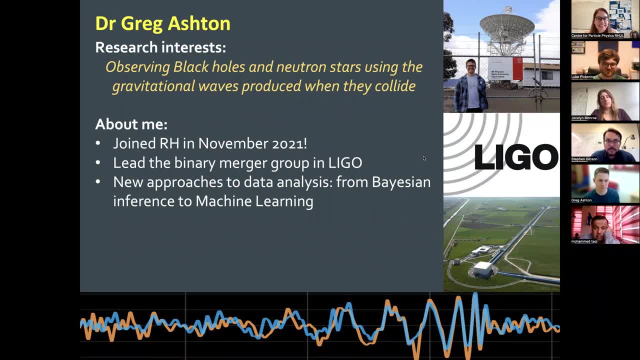 particles and lots of exciting things going on. Now I can take you from particles to waves. So we're a recent addition to the particle group. here We have a gravitational wave astronomy group and so a bit of background on me. So I'm a gravitational wave astronomer and really what I 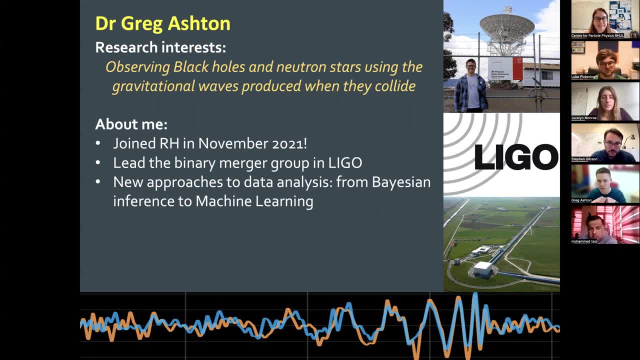 like to do is to observe black holes and neutron stars using what are called gravitational waves produced when they collide. So Einstein's theory tells us how gravity works and as part of that, it tells you that when massive heavy objects smash together, they produce little ripples in the fabric of space-time, and those we call gravitational waves Now over. 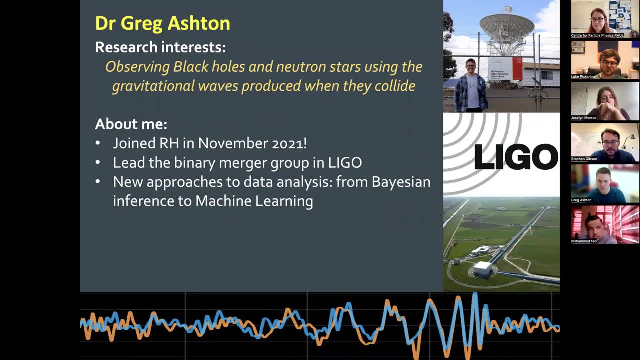 the last several decades there's been a development of instrumentation to detect those signals and in 2015, the first detection was made by the LIGO detectors. I'm a member of the LIGO collaboration and lead one of the working groups which studies these binary merger. 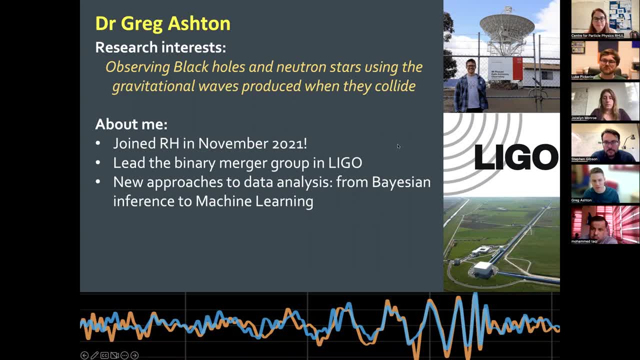 collisions. I'm a member of the LIGO collaboration and lead one of the working groups which studies these binary merger collisions, So the group really kicked off here in November 2021.. It's myself, we have a PhD student and we're looking for more to join us in studying this and the kind of research that we are doing here is. 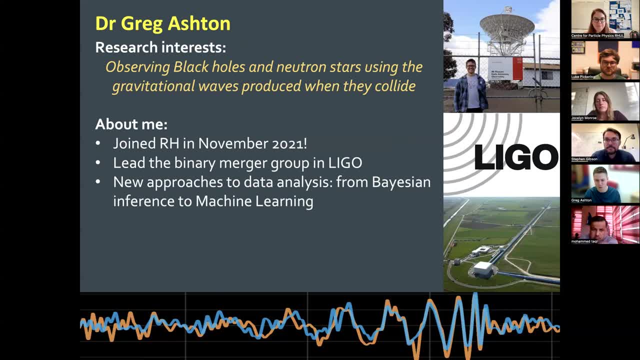 really about the data analysis side of what you do with that data. So down at the bottom I'm showing the actual gravitational wave itself. so you can see two sort of tracks overlapping one another and there's some wiggling back and forth and what you're seeing? there is two. 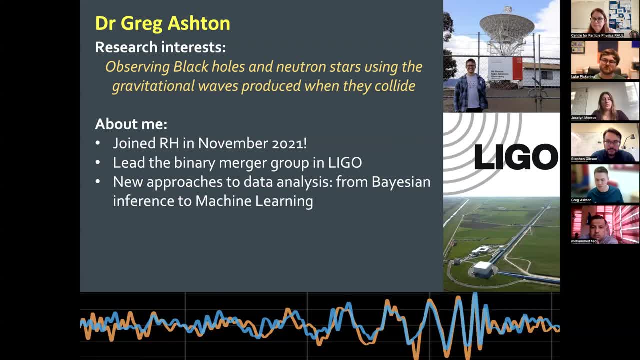 black holes rotating around one another and as the frequency increases, that's as they get closer together, and then you get a sort of largest amplitude as they collide together, and then nothing after that, and so our job is really to take that data and learn. what does that tell us about the 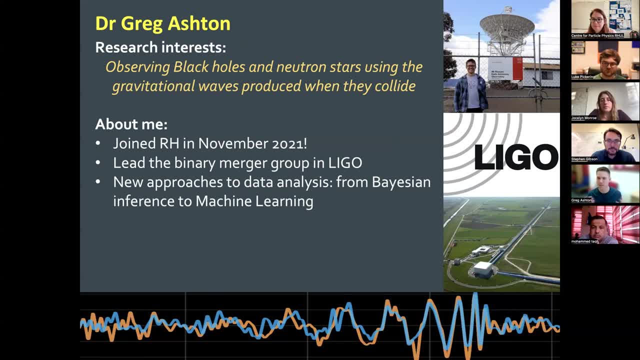 black holes, and also about the properties of the universe and how it's evolving. So there's three projects that we're looking- or one of three projects that we're looking- to fulfill for the next year. The first is in what that data can tell us about Einstein's theory of relativity and if there are, 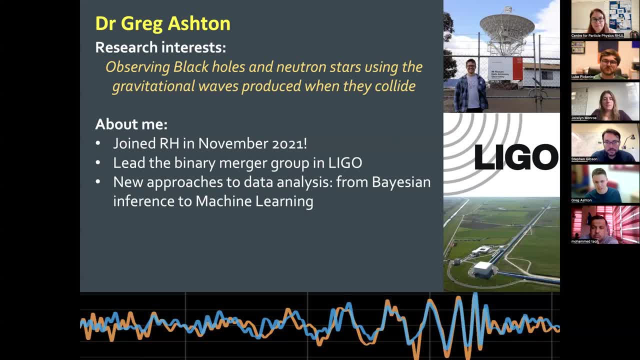 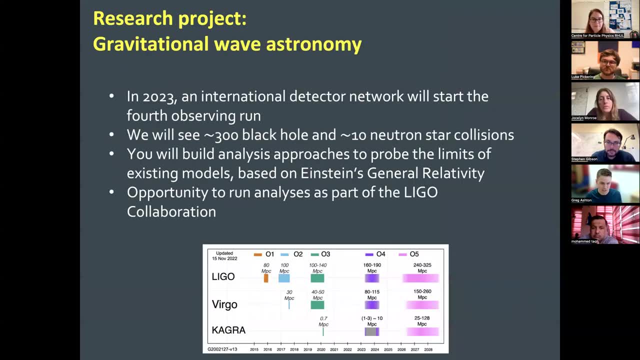 holes in that theory and if we can probe them. The second is about using advanced artificial intelligence approaches to actually study that data. So traditionally, we've used what are sort of known as sampling algorithms, and what we'd like to do is to improve on that with things like 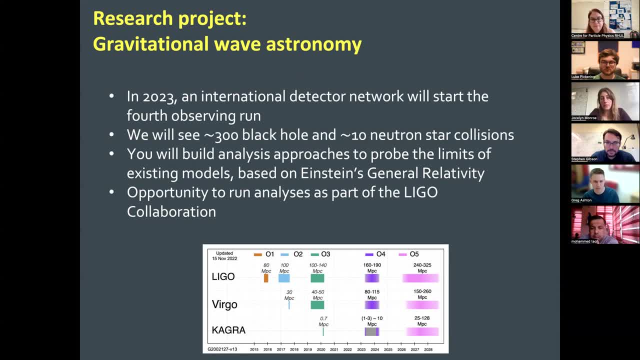 machine learning and collaborate with some of the colleagues from the computer science department here in rural Holloway to do that. and the final one is to look at the properties of the noise and see what that can tell us. So, moving on to this slide then, what would it? what would? 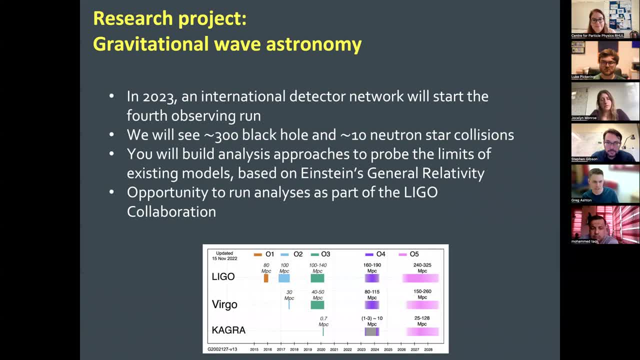 it look like in the sort of timeline of a PhD. So as of next year, the international detector network will start our fourth observing run. so there's a little timeline down at the bottom there, and so you can see. LIGO started in 01, in 2015 or so, and that's when the first detection was made. 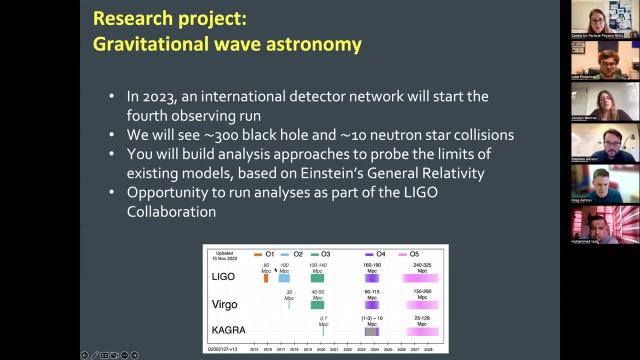 since then, we've had three observing runs, so the most recent finished in 03, finished in the middle of 2020, and there's been a very long, extended gap since then, partly due to COVID, but mainly because the scientists have been busy improving the detectors, and so what's quite exciting is in. 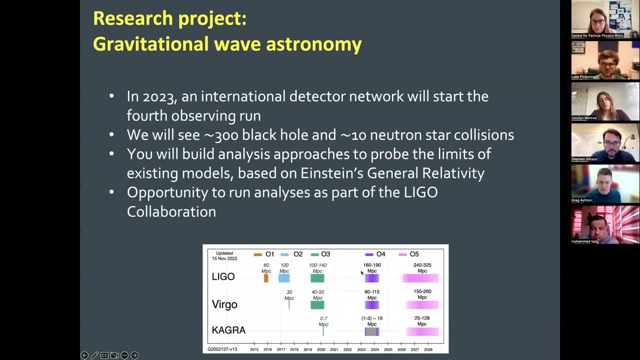 April next year the detectors will switch on- not only the LIGO detectors, but they're joined now by the Virgo detector in Italy and the Kagura detector in Japan, and together they'll see something like 300 black holes in a year. so that makes it something like a black hole per day. 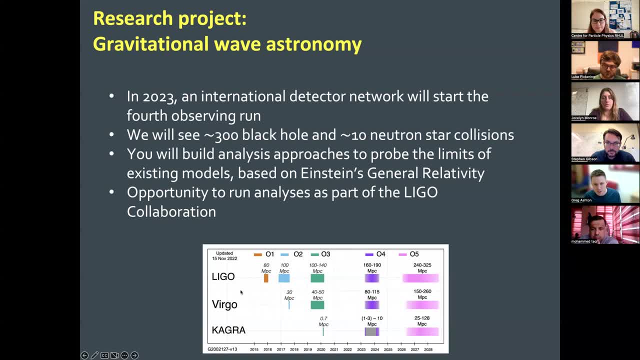 and also 10 or so neutron star collisions. So the PhD will focus on building analysis approaches to probe the limits of these models and Einstein's general relativity, and there'll be opportunities to sort of run those analysis as part of the LIGO collaboration and contribute to that 04. 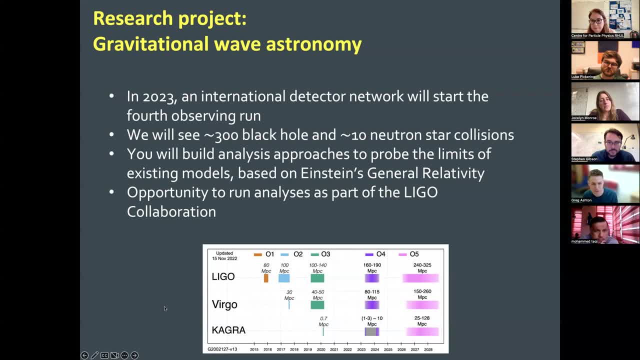 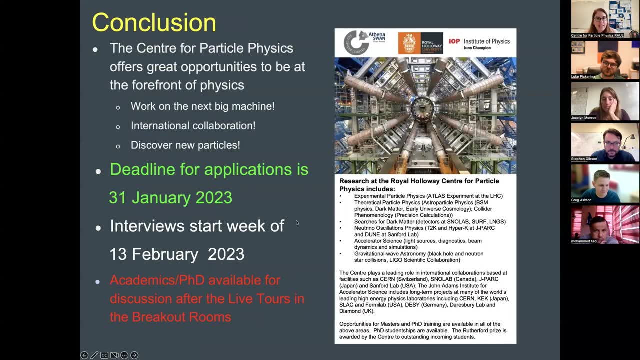 observing run and and the analysis that follows. So I'll finish up there and pass back to Ronnie. Great, thank you. so much very exciting stuff coming up. Good. so here's the conclusion. so hopefully you've heard about all of our great opportunities to work on the next big experiments. 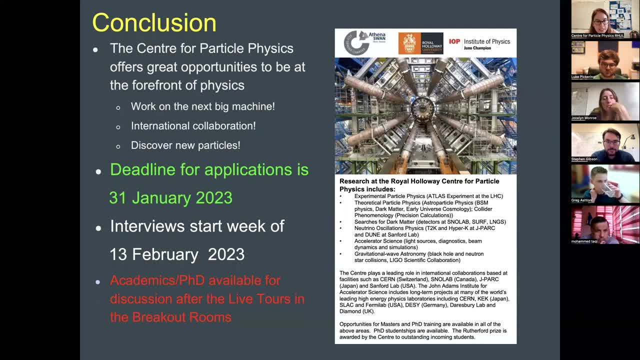 and theory. Our deadline for application is the 31st of January 2023, and so you can find a link to the application form, which is an online application form, from our physics opportunity page- PhD opportunity page. If you have any questions, then, of course, you can get in touch. 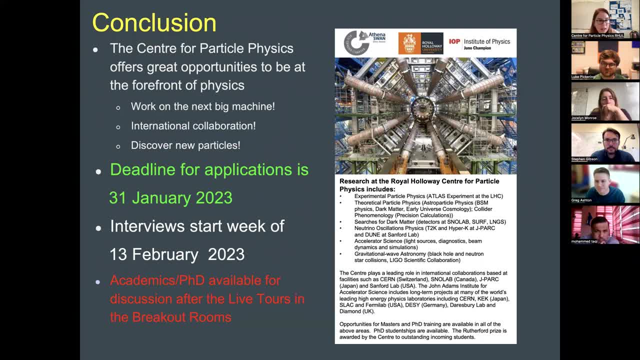 with me and I can help you find the right link. We expect that the interviews will start around the week of the 13th of February and you'll hear more about that after you apply. So there you go. so if you have any questions, we can take some Now. the idea is that we will get some live tour from some. 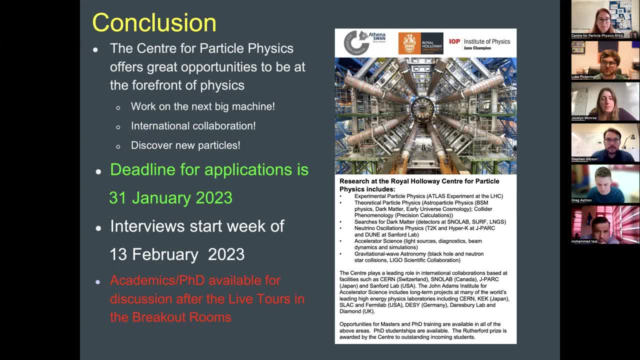 of our speakers and then we'll have a little bit of a chat, and then we'll have a little bit of a discussion and then after that we will open the breakout rooms and then you'll be free to go from one room to another, whoever you want to talk to, and it's very sort of free, it's very informal. 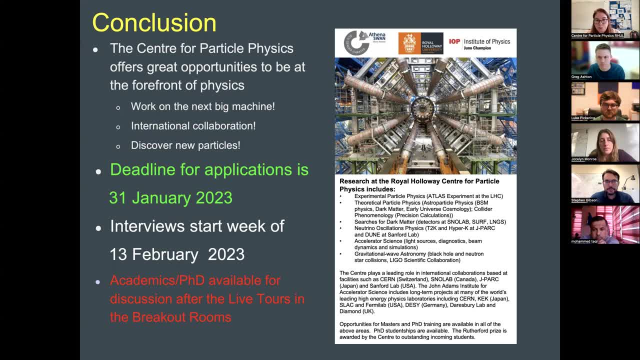 and that would be the the end of the event. and so once you've had all your questions and your discussions with whoever you want to talk to, then you're free to disconnect and and that will be the end of the event. Okay, so I don't know if there are any. 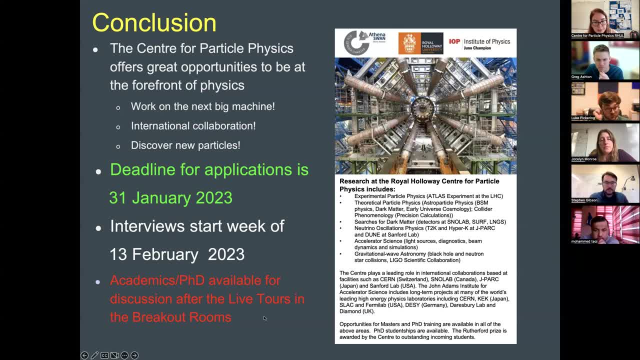 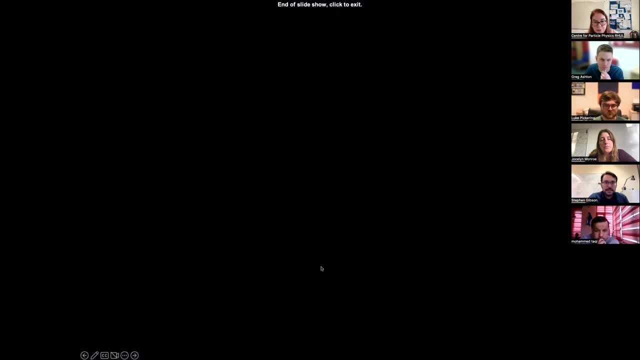 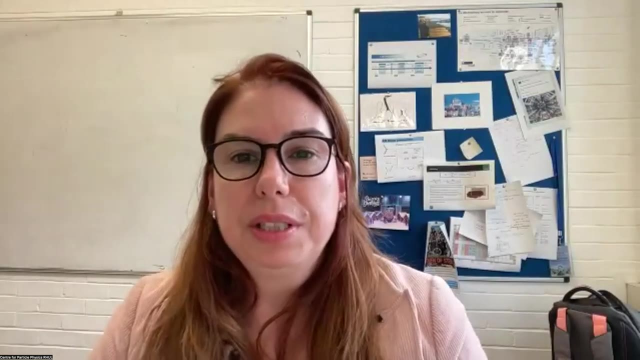 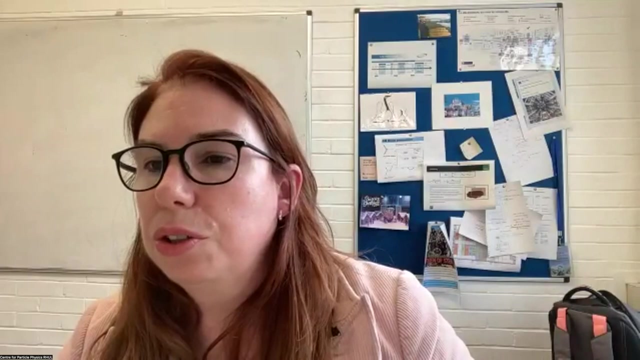 questions. urgent question at this point. if not, then we can start with the tours. So I'm going to stop sharing and there we go, there we go, and so I think we have Professor Gibson giving us a tour and also other activities here, and so I don't know who would like to start first. 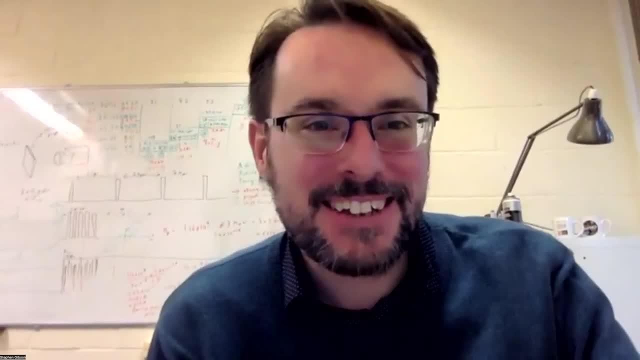 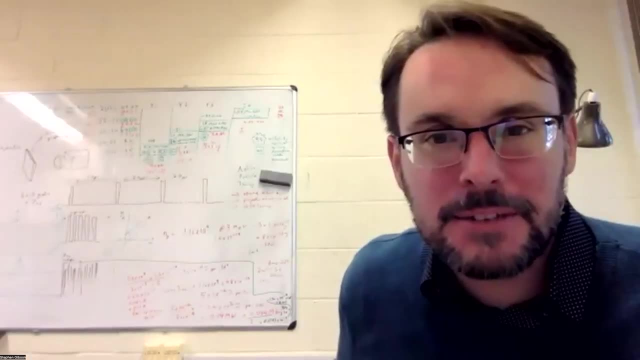 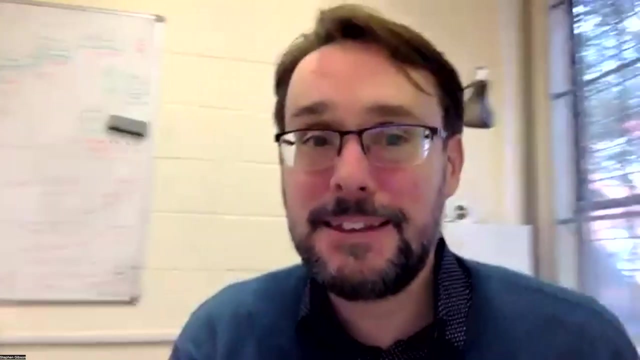 I mean I can take you from a tour from the office to the labs, if that, if that would be useful. Where are the other tours? are they up in the next? I think they will be up. yes, Okay, so maybe if I I can walk you past the LaserLab and then up to the DarkMatter Lab. I think that's right. yes, 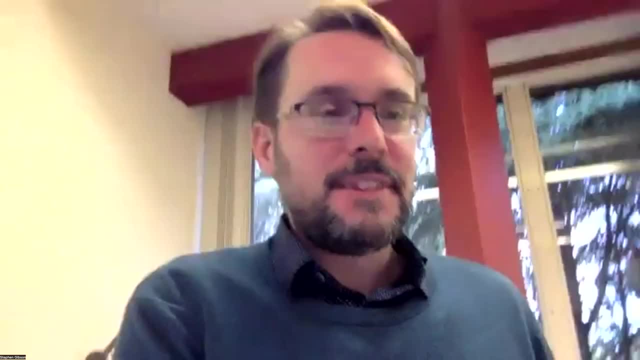 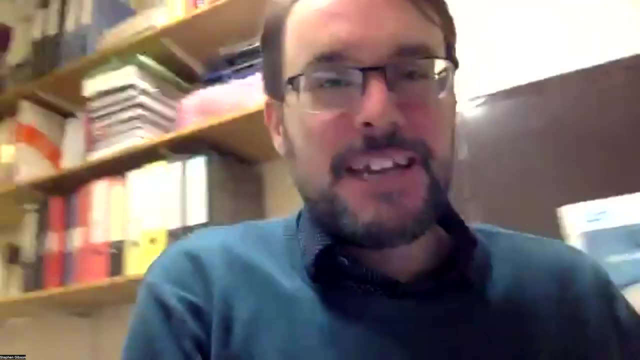 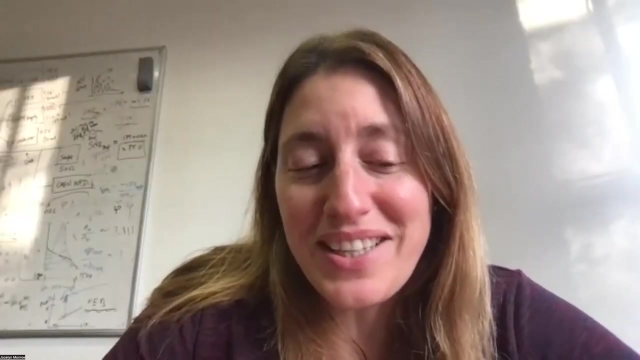 Good way to go. okay, so I'll. I'm currently walking with the laptops. hopefully the wi-fi will remain intact as we walk around the building. but let's also Just to say Ali is in T133, so he's right next door to you. Oh, brilliant, okay. well, let's pop in there and see that space. 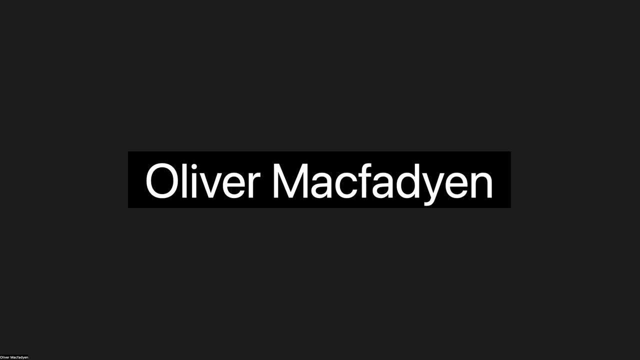 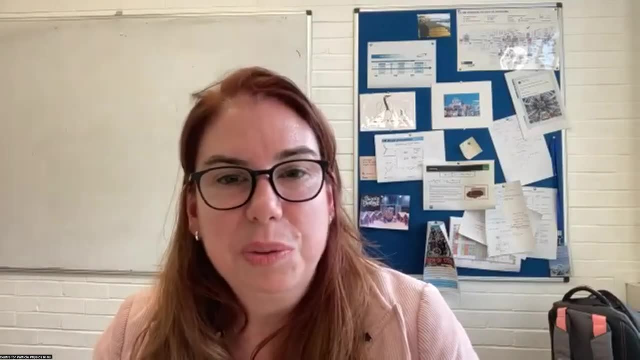 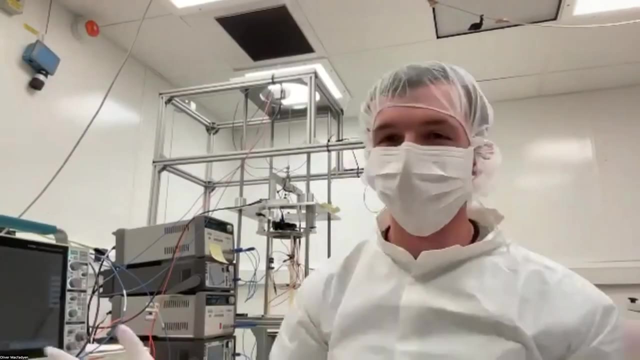 I can. I can take it from here. I'm already inside the clean room, if that's any help. okay, so how about we start with you, Ollie, and then, uh, Stephen will sort of go to his lab and get started. hi, we can see you. that's excellent. so, okay, this is um, this is one of the dark matter. 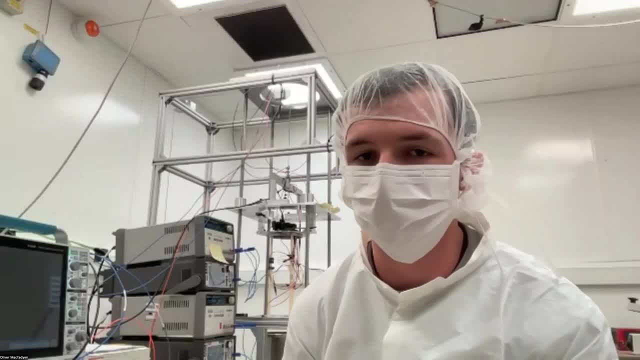 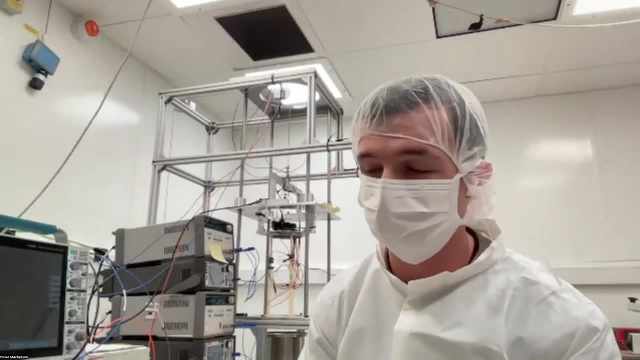 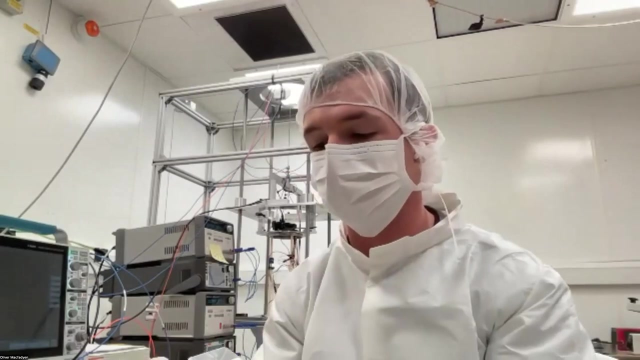 labs that we have. so this is our clean room that we have for um, for dark sides, 20k. so I'm one of Jocelyn's PhD students, um. I'm in my second year and I've been working predominantly on the testing of the little photo detectors that Jocelyn mentioned in her presentation. so 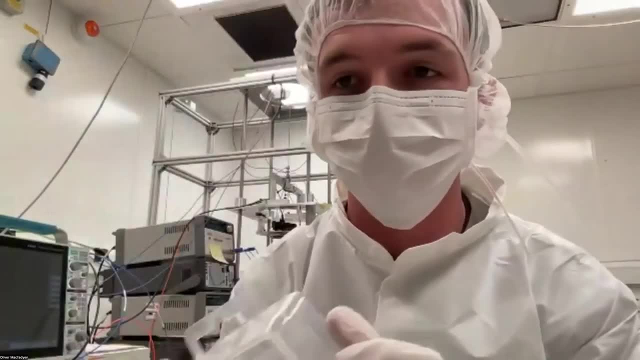 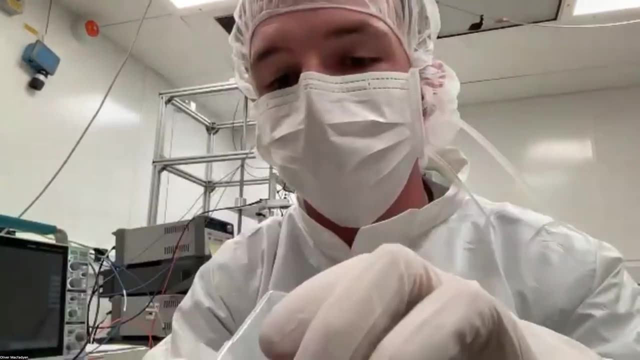 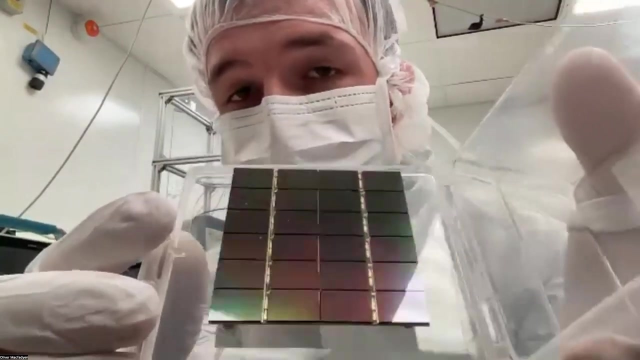 I've got one here and I'll hold it up to the camera it is. it's quite small, so they're only five centimeters by five centimeters. so, um, these are the back end electronics. and then the most interesting part is, uh, it's beautiful silicon that we have on the front. so, um, these are 24. 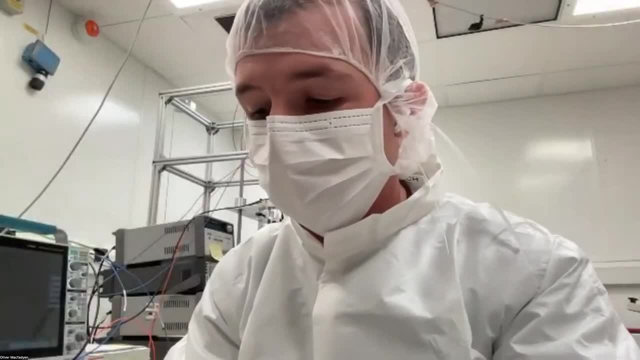 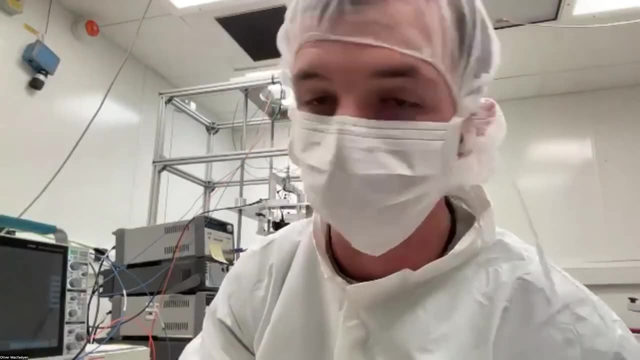 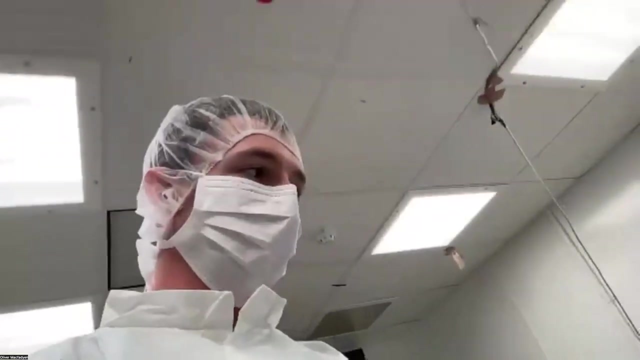 meters and um. what we do, um here in our lab is that we test that we can get um single photon efficiency, um single photo electron efficiency on these side PMs, um. so what we do, I'll just take you over to our little test stand that we have. so this is our, this is our test stands that we use to do. 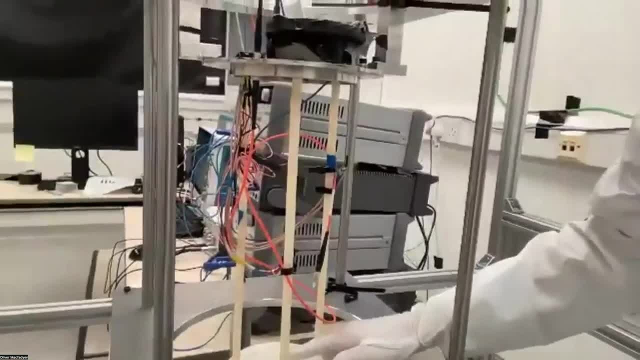 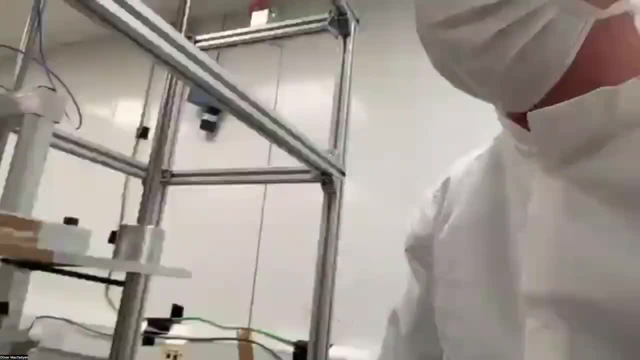 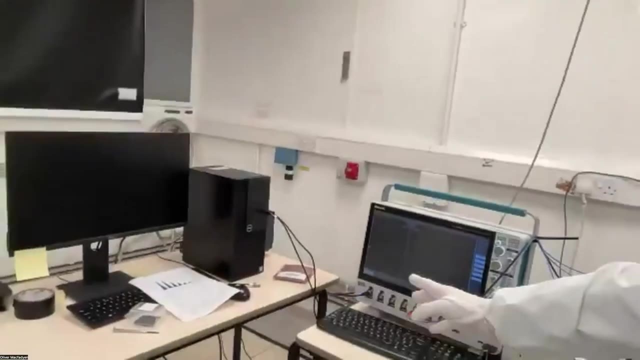 all of our side PM testing. so we mount the tile here on the test stand and we fire a laser at it to see and rate um. so then, um this, all this data gets outputted through lots of cables that we have um to our oscilloscope, where we can then record all the data. and we do this both uh room. 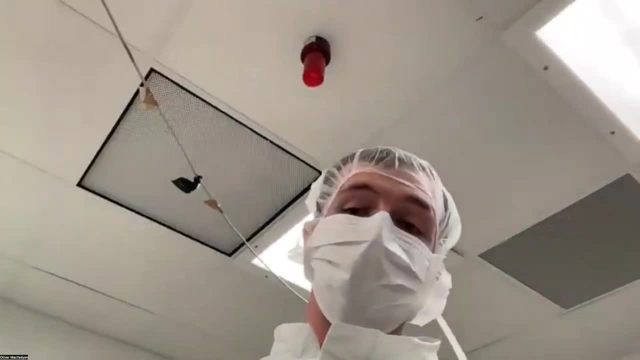 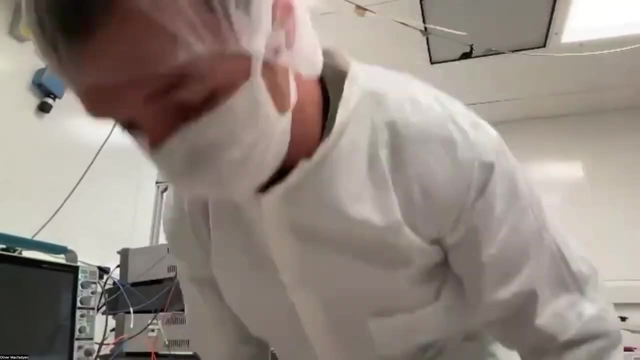 temperature, so about 20 degrees, and um liquid nitrogen temperature, which is quite fun. so, um, you get to play with some cryogenics if you join our group, um, and what we're aiming to get is an output that looks um, I don't have a slide prepared, unfortunately, but I've got. 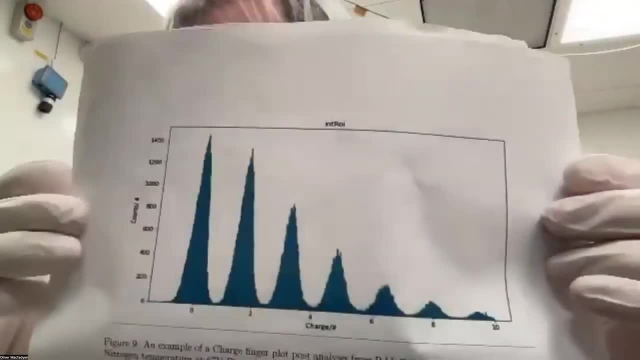 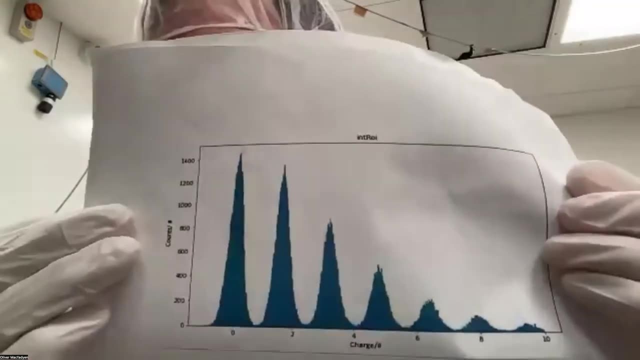 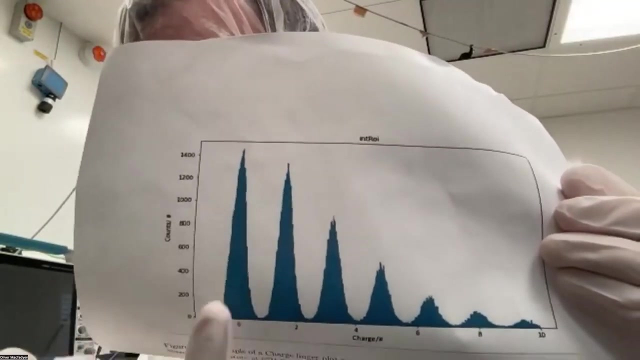 um, a printout of what it should look like. we are hoping for an output on our oscilloscope, or something like this. so this is what we call a finger plot, and what we get here is that each of these represents the number of photons you detect at a single time. so this is a zero. so 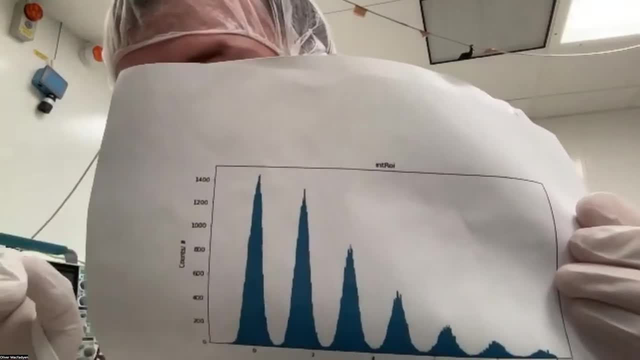 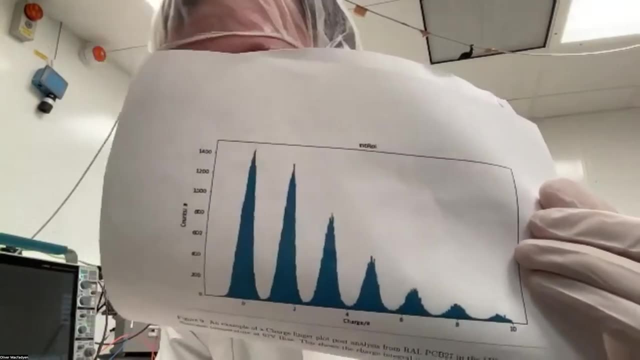 this is the amount of times when we look at our side PM and we don't see anything at all. this is where we look and we've detected one photon, two, three, four, five, six and so on, um, and what's really cool about this is that, um, it literally can be that precise, which is pretty. 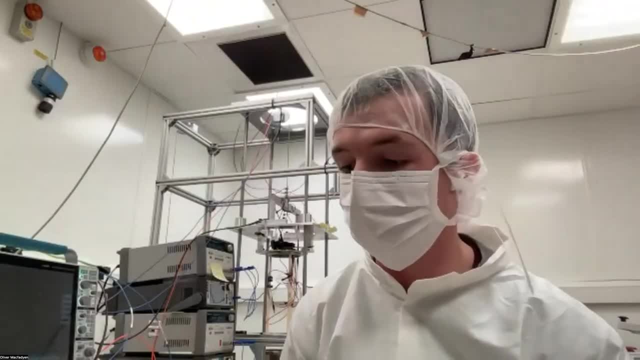 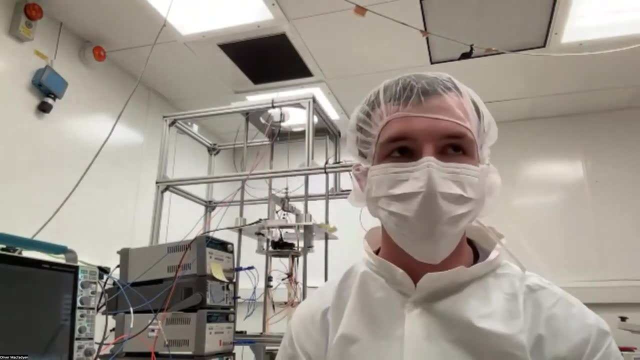 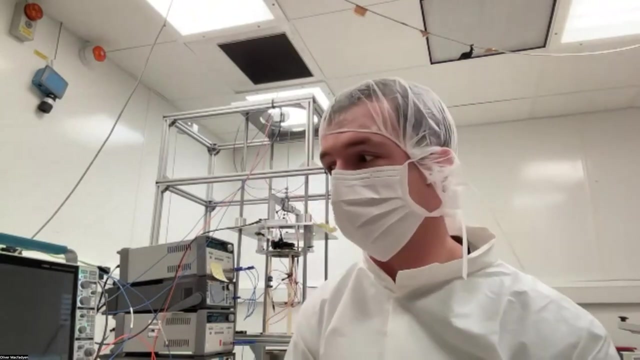 amazing, um, and what we've been doing is that, um, we've been testing the first few production runs for dark side, um, so we've now tested, oh, between 25 and 30 tiles. um, constantly modifying our setup and improving it, and now we're we're just coming how about halfway through a second test run about. 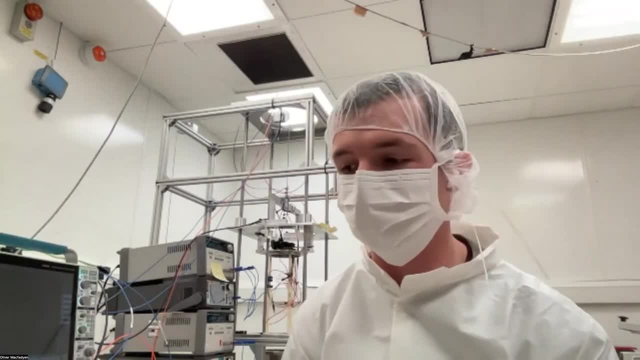 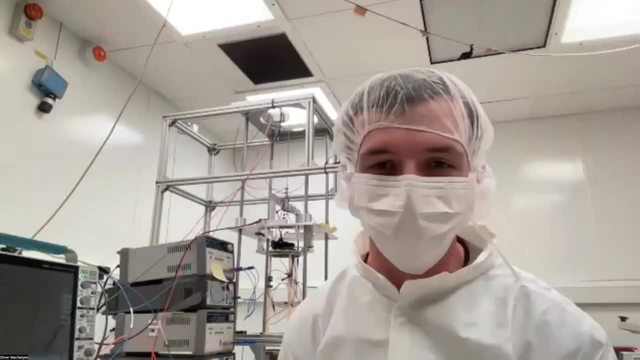 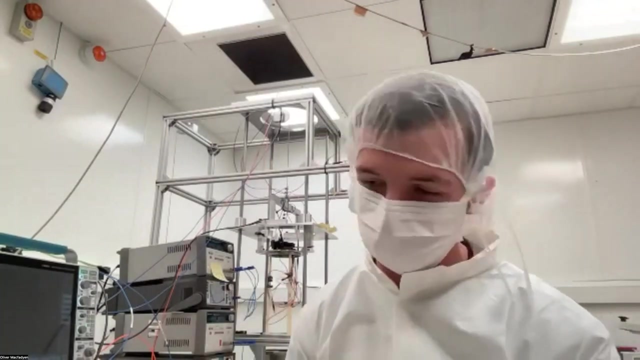 a test run, with each one being about 16 tiles. so, uh, one thing I can't say about the dark matter group is that it is- it's the best of both worlds. you get to do a lot of analysis and stuff like that, but you also have an opportunity to do a lot of hands-on work and hands-on experimental physics. 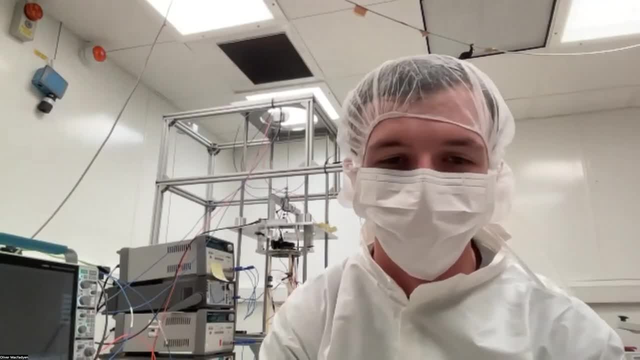 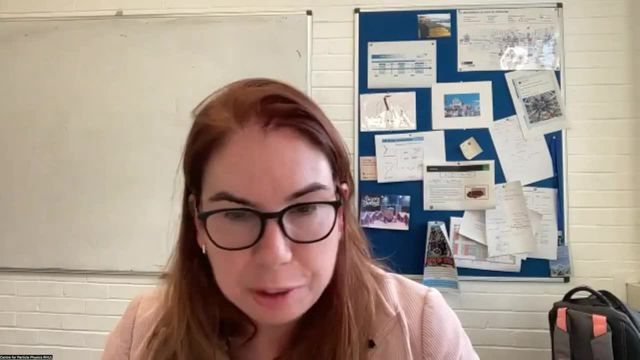 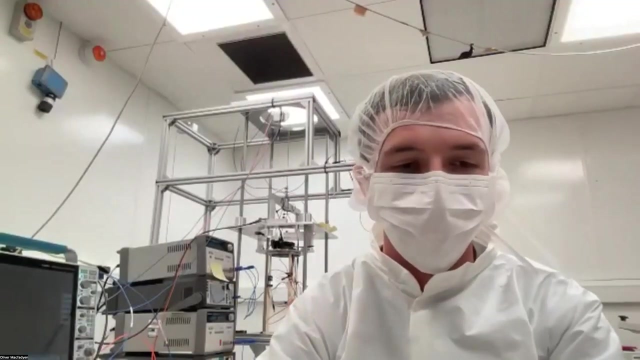 which is very cool, great. thank you so much. very good, and um, I think maybe you'll be in the PhD room later on, or at least some of your colleagues. yeah, yeah, I'll, I'll be. you know, I'll be moving over to the room later, that's right. so if anybody has question, 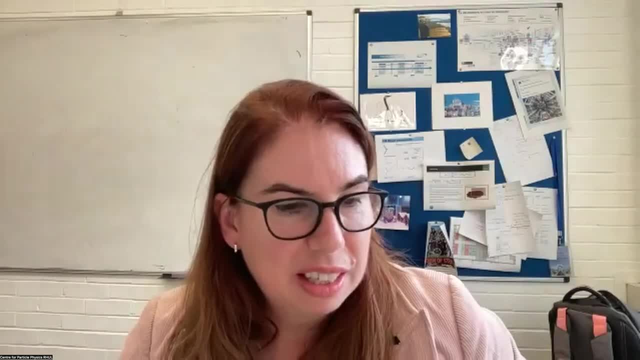 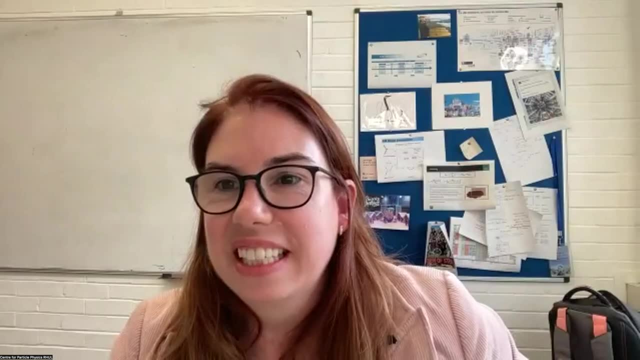 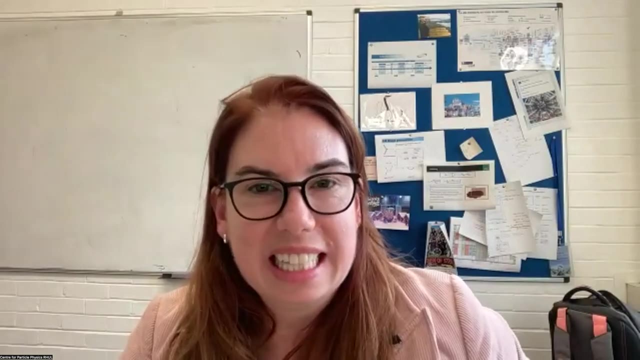 about either the setup or what it's like to be a PhD student in this group. then you can discuss that great. so thank you so much, Ali. uh, very exciting, and uh, maybe we can go back now to there. you go to Stephen who's in his lab, so feel free to take it away there. 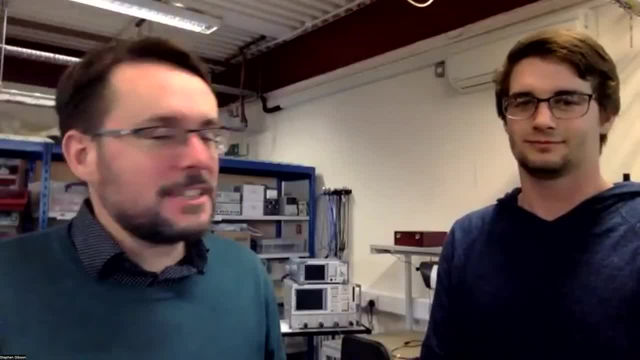 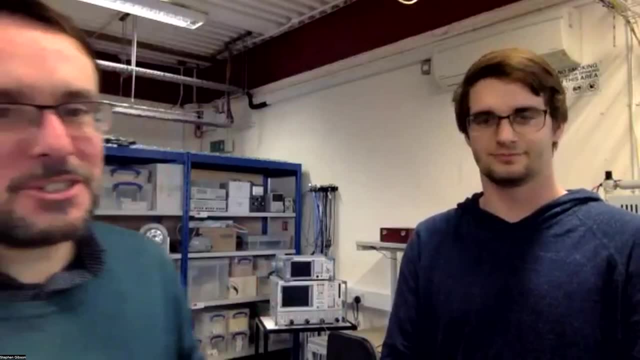 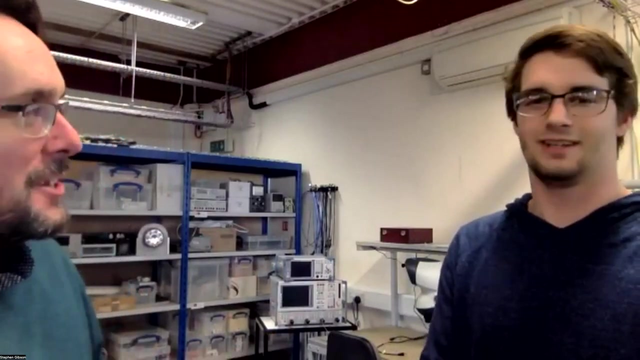 um, okay, thanks, uh, Veronica, great, great to see uh t1233 and um, so let me introduce you to Mark uh, who is working here within the John Adams Institute. uh for its analysis, science and working on, well, RF electronics and developing our sources. I don't know, Mark, would you like to say a bit about what? 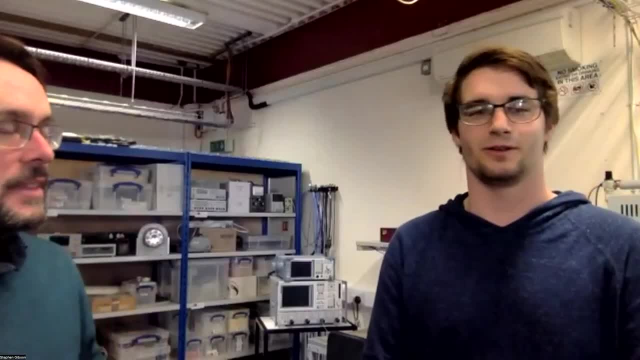 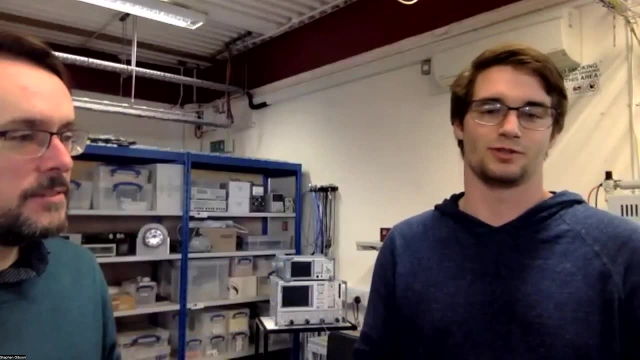 you're working on. so for the last year I've been working on um designing and developing a sort of family of compact high frequency radio sources. um, they use modular components which you can. you can use modular components which you can use, modular components which you can basically like Lego, just um placed together, and I've been working the control behind that and 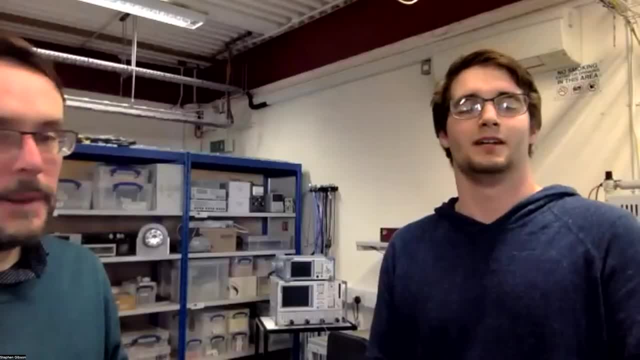 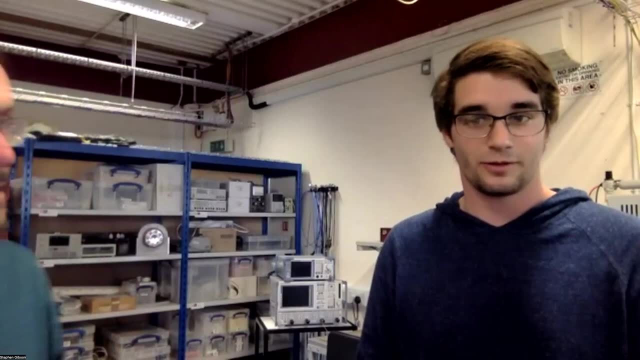 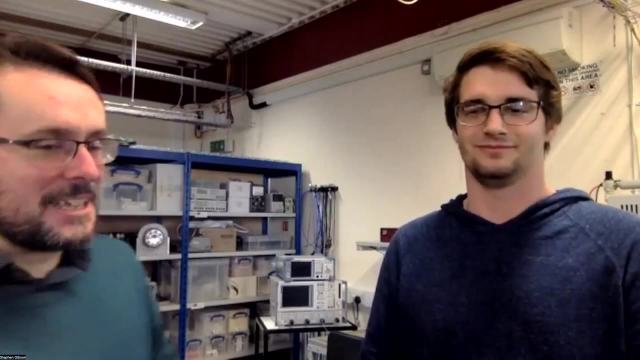 using micropython, so coding a lot of python. um, I presented my work at a conference in ibik, so I got to travel to Poland, which was quite nice, and I should hopefully be starting my PhD in January. so, um, yes, what I've been up to, yeah, yeah, we look forward to you starting there. so just to just 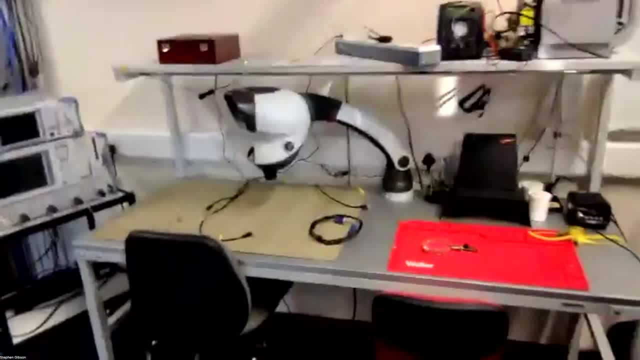 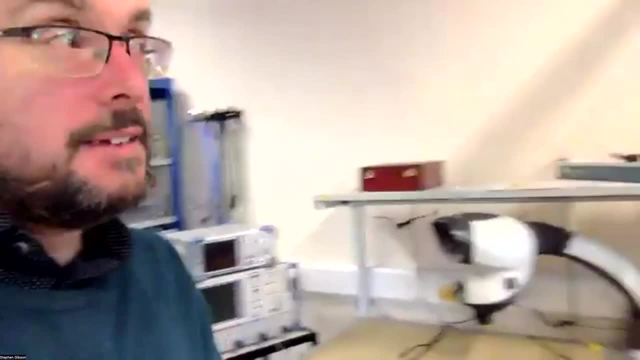 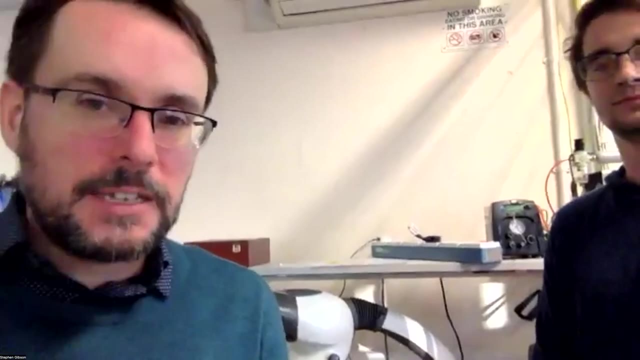 uh to show you a bit around the lab. um, you know, we have uh some equipment here, so this is mainly uh for testing RF electronics. so radio frequency electronics, where you know we're the accelerator, has basically a heartbeat that provides the pulses that go through the accelerator chain and so that heartbeat is really fast. it's normally hundreds of megahertz, and so having electronics that operates at that speed is really important. and if you want to measure the shape of those pulses, you have to go to even higher frequencies- a gigahertz or tens of gigahertz- to be able to measure such frequencies. 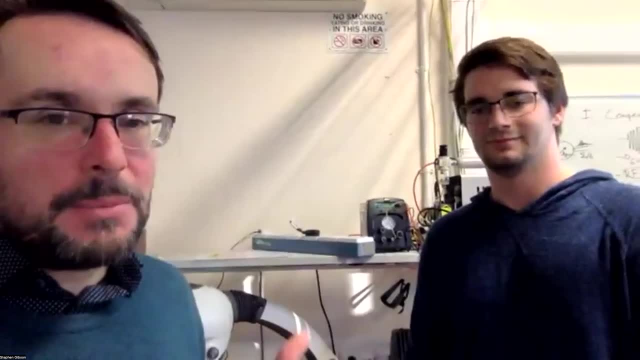 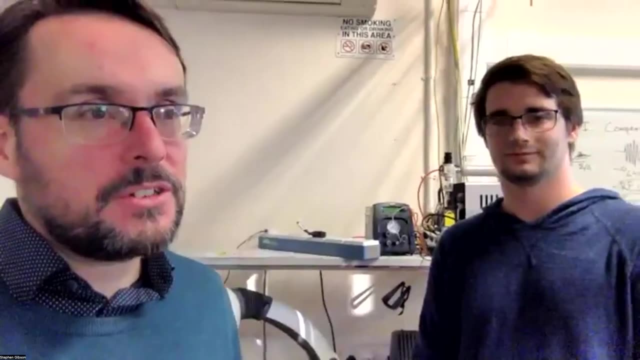 so having, uh, these sorts of skills, developing those skills throughout your PhD is, you know, really valid and important thing to do in this field, but also in other fields. so taking your research and then moving on, for example, to to telecoms or photonics, you know we often use. 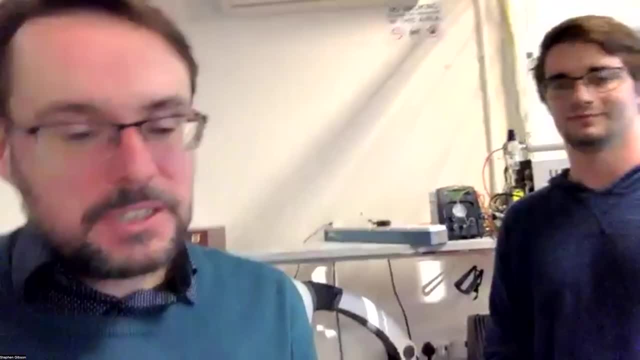 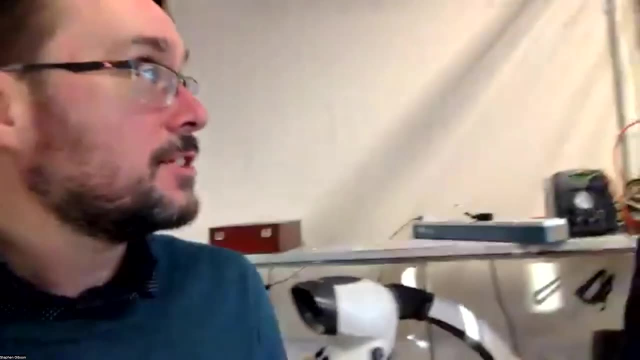 really high uh frequency uh devices like a. I've got a vector network analyzer behind us, for example, which is a common uh thing to use in in that kind of research. yeah, I've used the vector network analyzer and the spectrum analyzer quite a lot over well, so I think that's a good way to go. 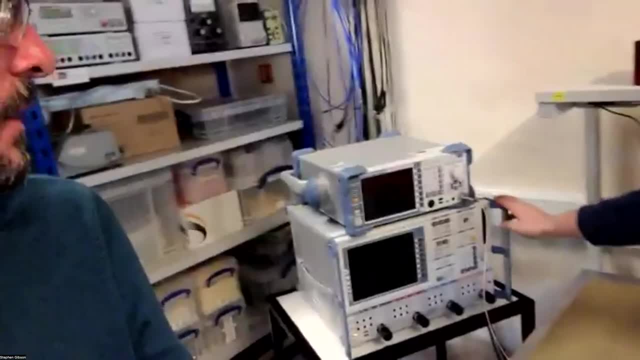 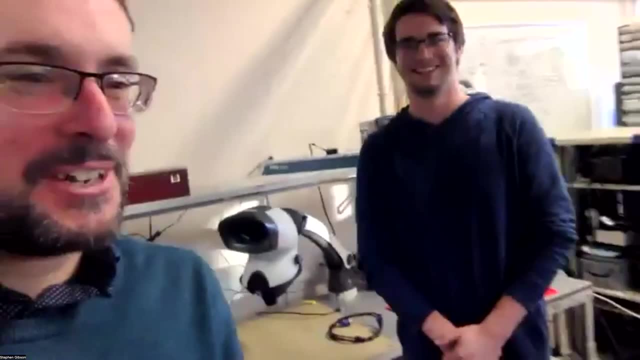 last couple- uh, last year, yeah- which is a vector network analyzer and a spectrum analyzer on top. unfortunately, they're not turned on at the moment. um, yes, okay, yeah, it's a bit of an ad-hoc calm tour, I'm afraid. so for that much. um, what, what's this down here? do you want to show you? okay, so this. 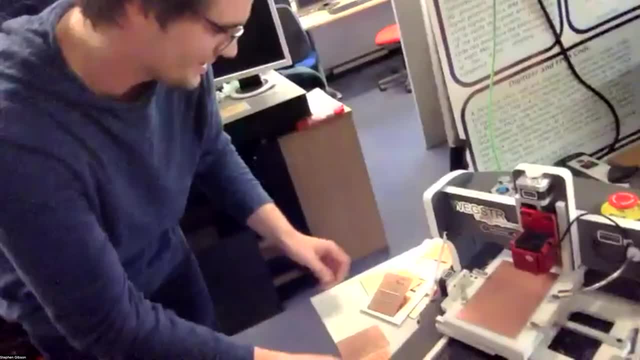 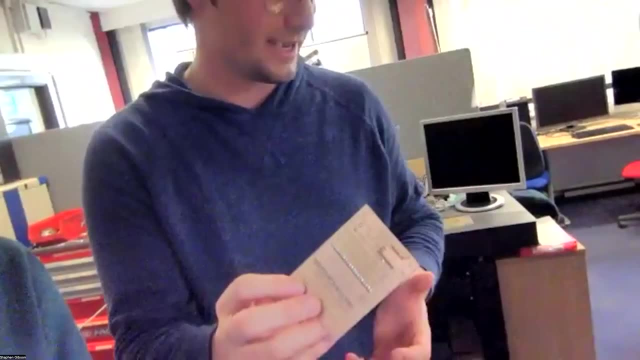 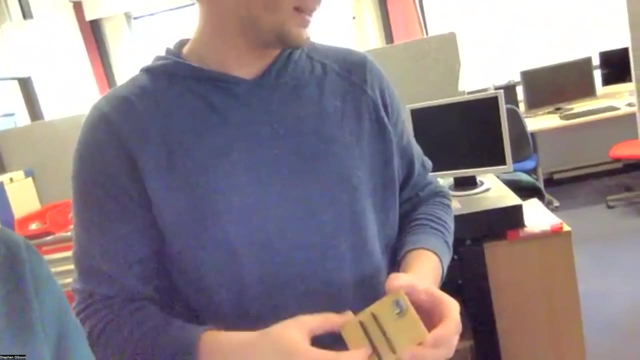 is a milling machine and what we've been trying to do is design our own PCBs, uh like this, and use a piece of software called KiCad and the whole point of this is to house sort of the electronic ranks for my sources. um, we had students use this machine over summer and we had a summer student. 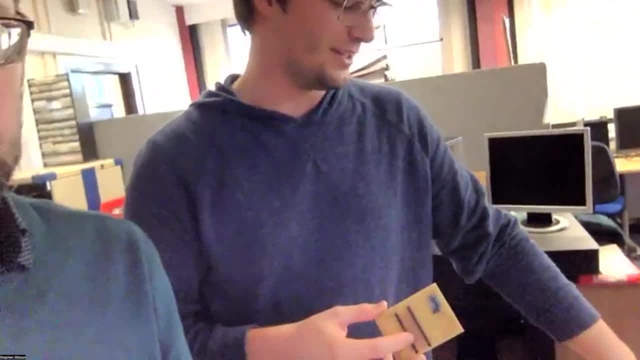 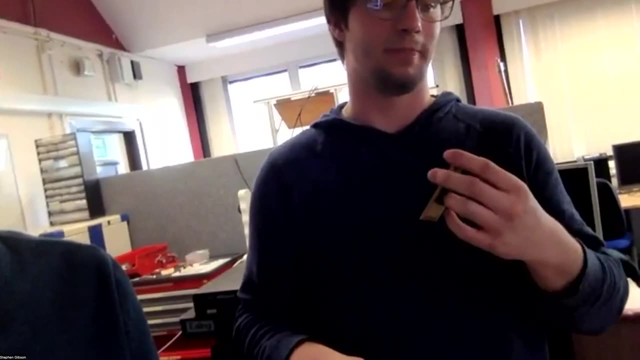 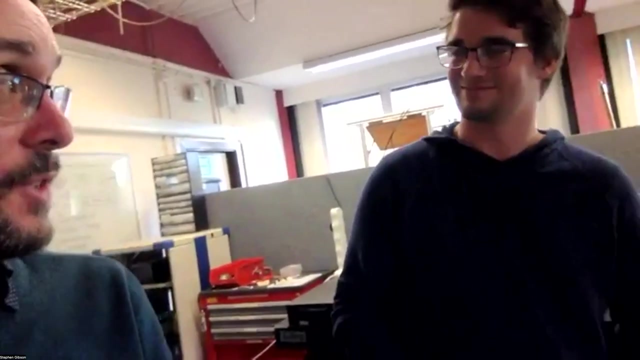 Matthew- I think I saw his name in here. he was using the CNC machine to produce a PCB similar to this that's going to be used for a um, um frequency synthesizer at sound. basically okay. so um, yes, awesome, okay. thank you, Mark. I don't want to take too much of uh, overall tourist time, but 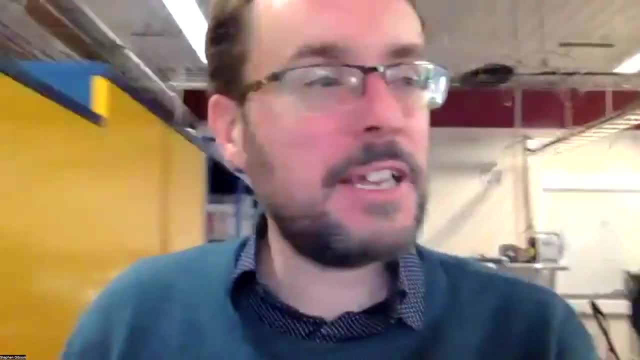 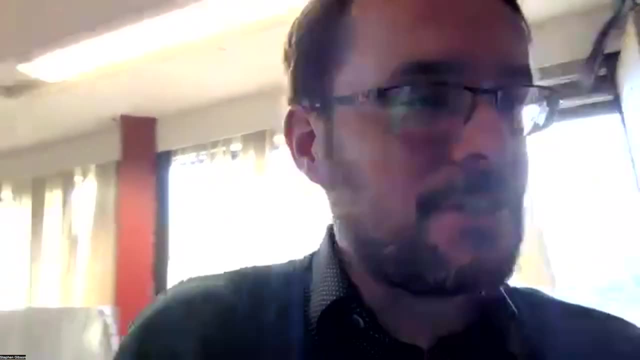 thanks a lot for showing us around. uh, I'm not sure where we're going next. I I do have a laser lab downstairs where Alessio is, so I could wander down there. or if you want to switch back to somewhere else while I move, that's also also. 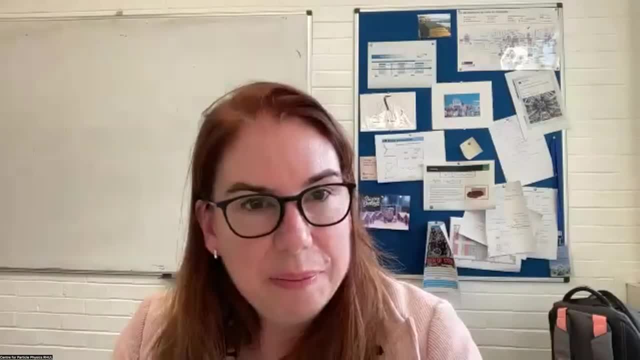 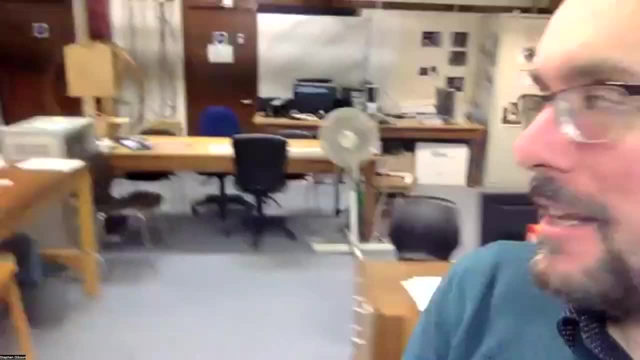 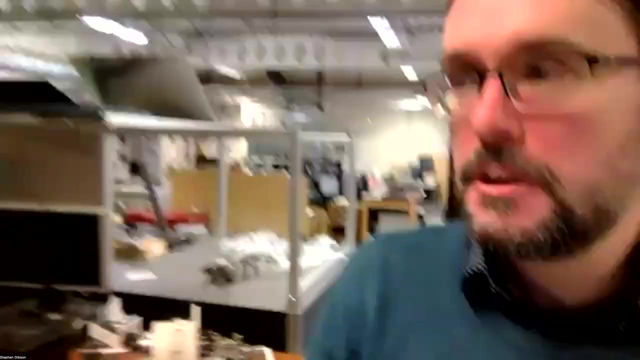 fine, or did you have any other people on the tour? no, I think, um, I think we were just giving a taste, um, here of the of the various things, so I'm taking you through the dark matter lab now as well, in the background. so this is where, uh, the time projection chamber uh was built. uh, for example, for the dark 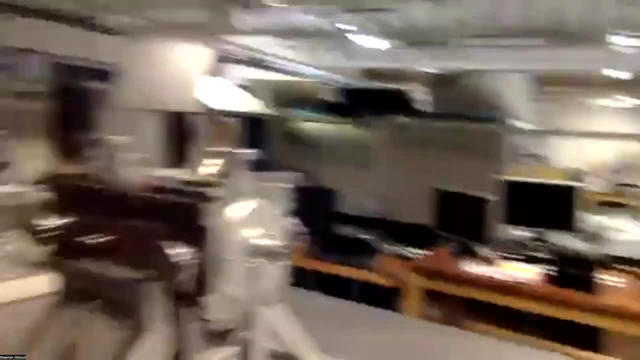 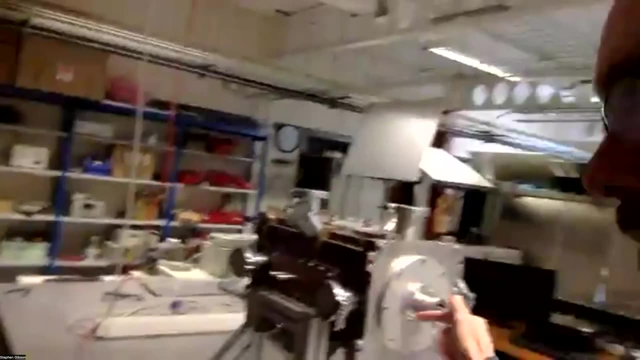 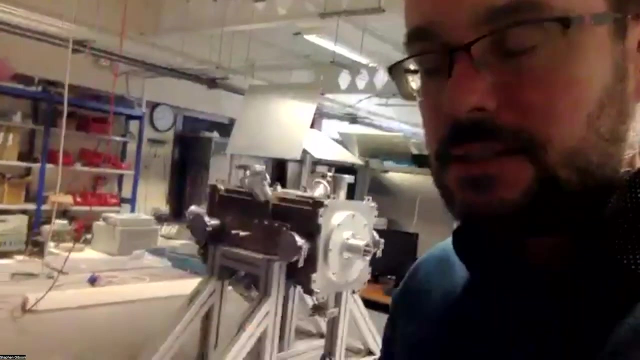 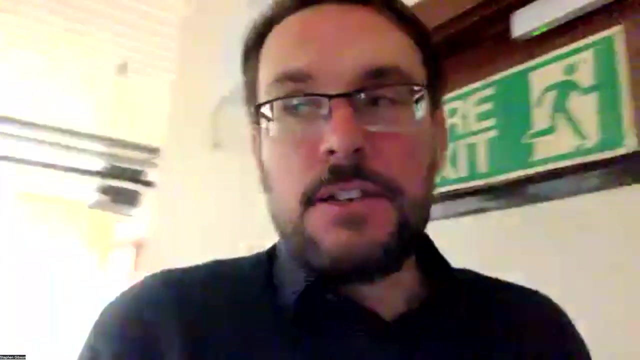 matter research. um, here is an actual little bit of an accelerator. so this is a radio frequency quadruple um of a short accelerator that's being built, or has been just built and first been tested this summer at the Rutherford Hamilton Laboratory. it's called the front end test stand over at RAL, so so 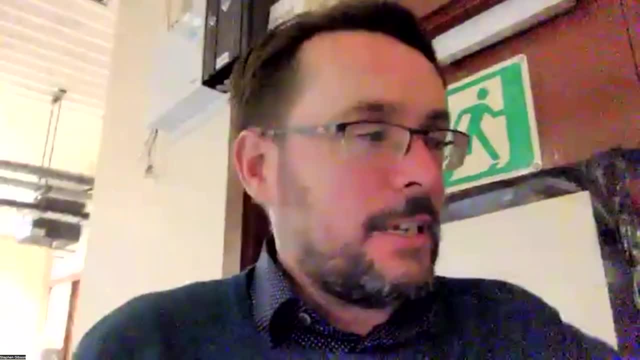 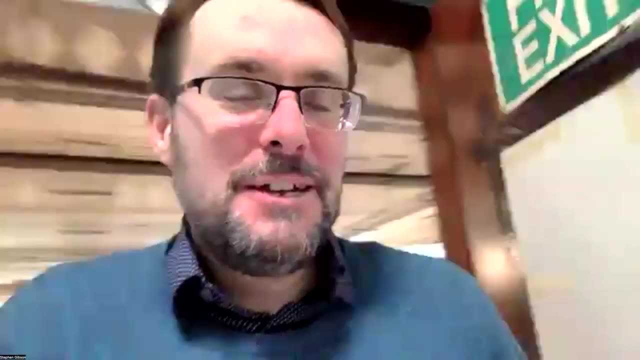 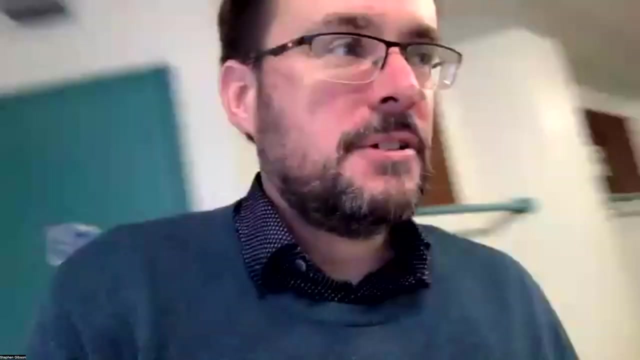 we've built the parts here and we've tested it and it's now an operating new accelerator for the UK downstairs. this is where the internet may become slightly unstable, so bear with me, but I'll take you out to the uh just down to the different area downstairs, and hopefully be able to get in the door. 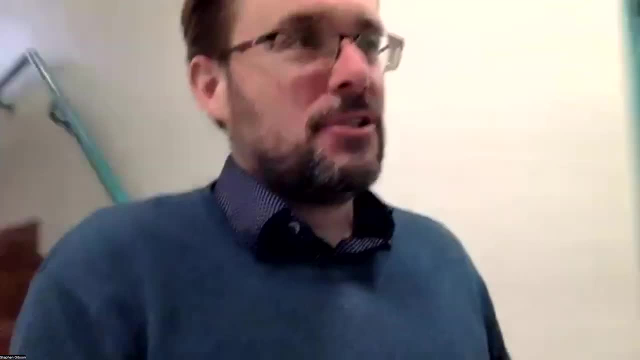 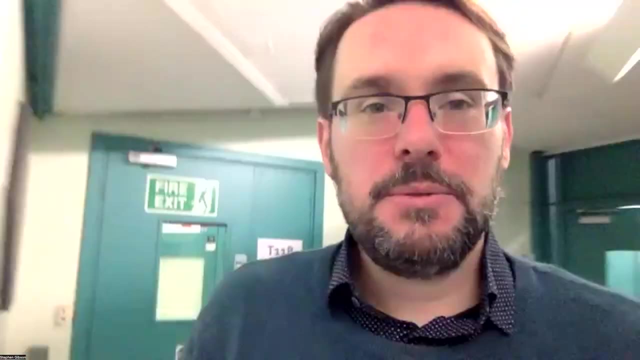 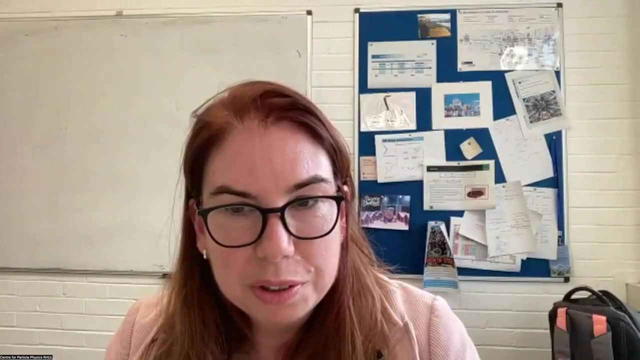 of the other lab which went slightly wrong on a previous tour. so let's see, let's see if we can find Alessio, who is in our other building. can you still hear me? okay, yeah, we can still hear you and see you. oops, you just froze, of course, but it will come back. 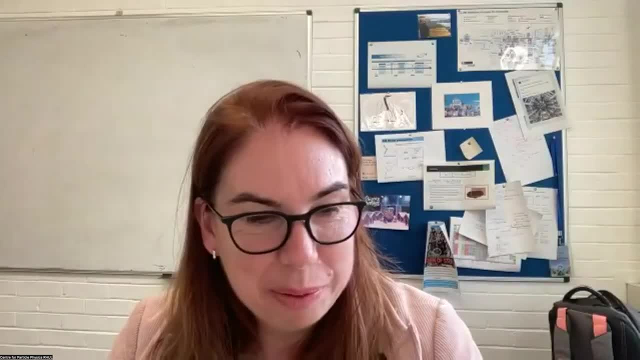 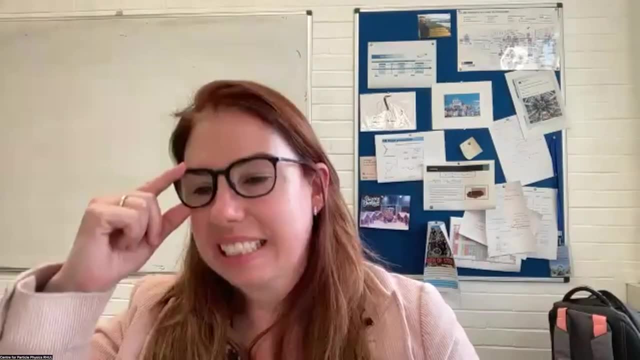 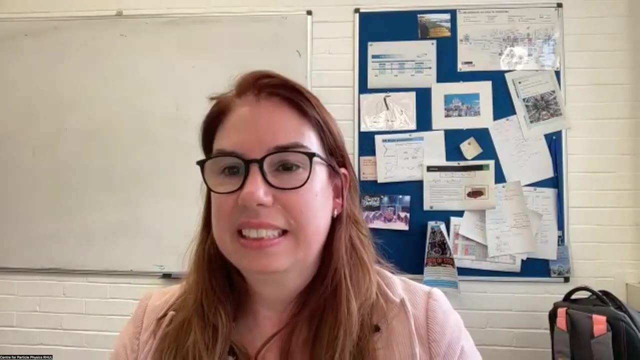 so I'm just um knocking on the door of our, our laser lab. uh, hopefully, uh, let's see, it was in there a few seconds ago. I mean, oh, there we go, it's just it's open. it's open, okay. so if we come through into here, let me just um. 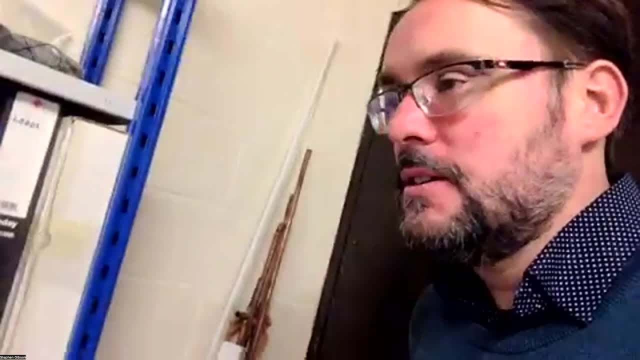 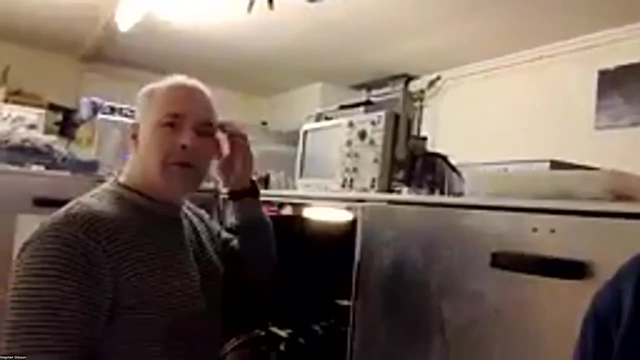 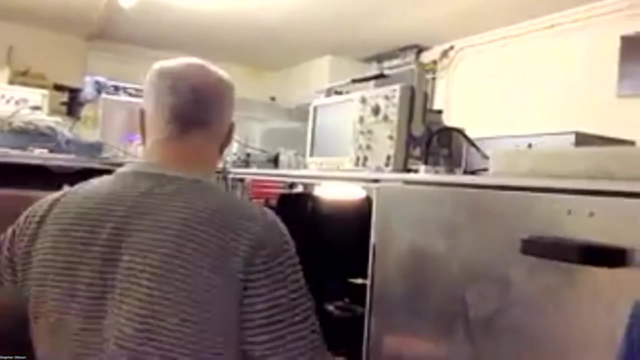 for safety. we've lost you a bit. yeah, there we go. that's our lab, where we do sort of develop a laser system or laser-based systems for accelerators, and so we can um. so maybe if you come to this side, the other side is better so. 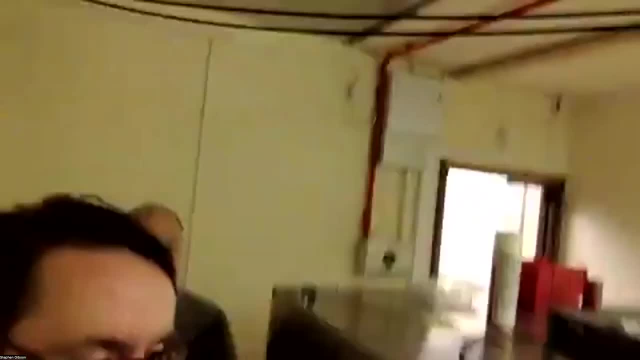 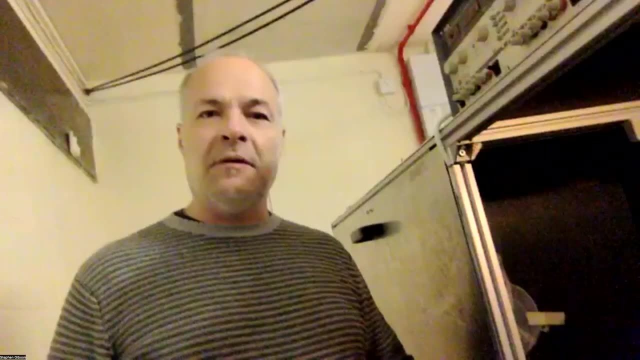 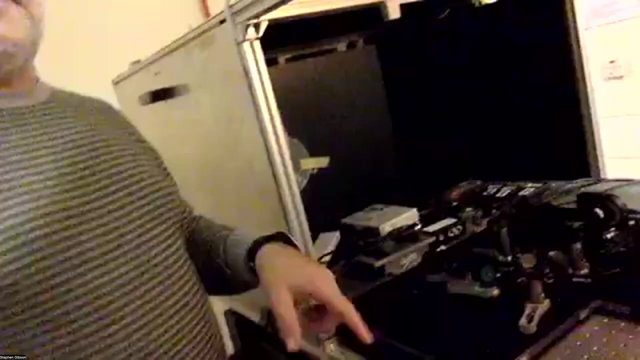 this is the- yeah, let's set up um for our laser wire system that we are going to be to be installing at uh, at uh FETS at the front of stands, and uh, at RAL, and it's uh, it's basically a two-dimensional laser wire system. uh, I don't know if you, they, know anything about it, but it's. 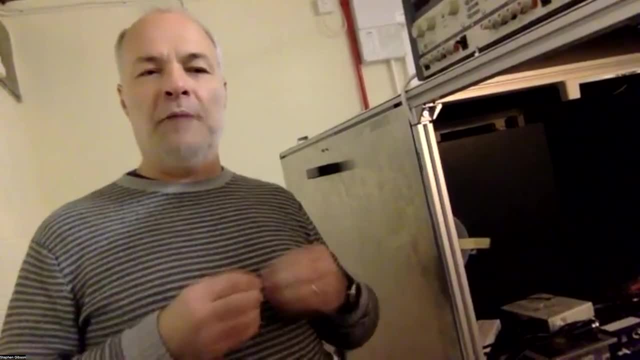 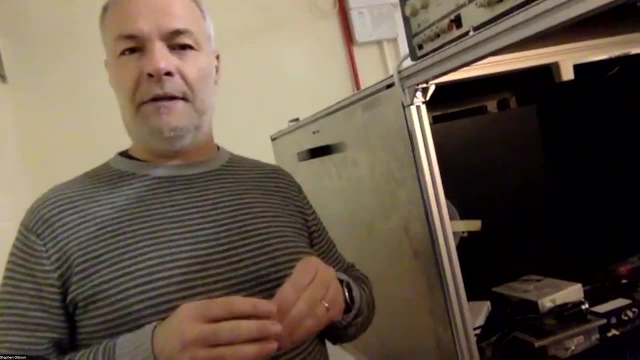 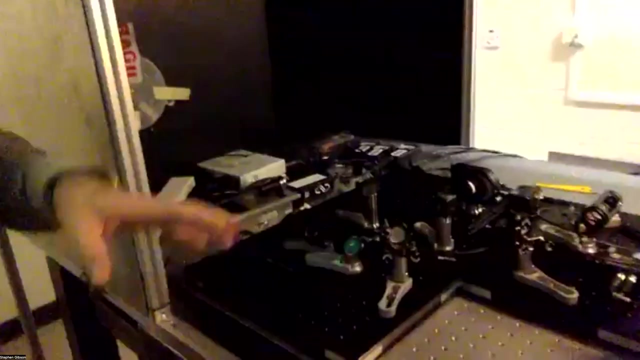 basically a system that we are developing, uh to, to be able to measure some uh, some um, H minus accelerated beam properties such as the beam size and the beam divergence or um. so basically this consists in a laser system, in a laser beam that it sends to cross the accelerator beam. 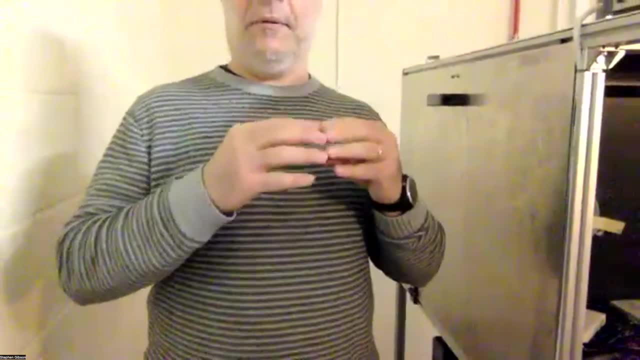 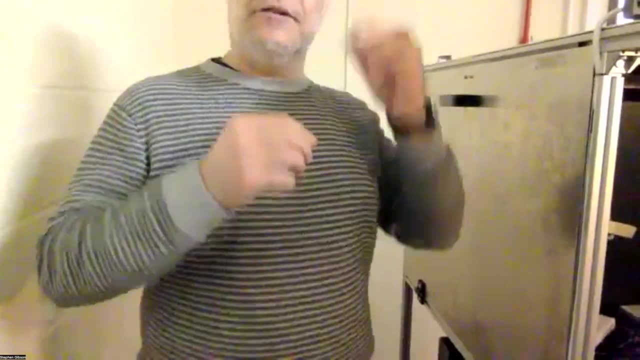 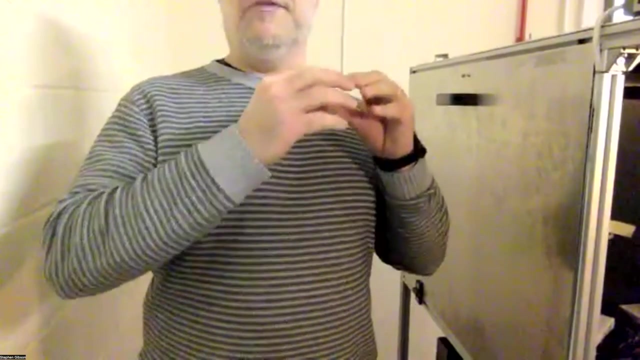 and and the interaction with the accelerator beam, which is made of aliens H minus science, or negative hydrogen ions which have an extra electron, and so the interaction with the laser will be such that the electron could be extracted from the atoms and then basically from the, the main H minus beam. we 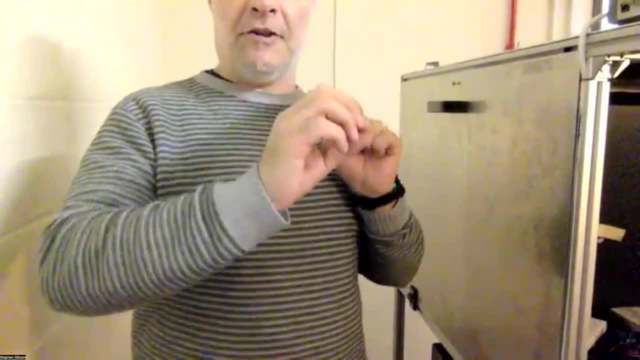 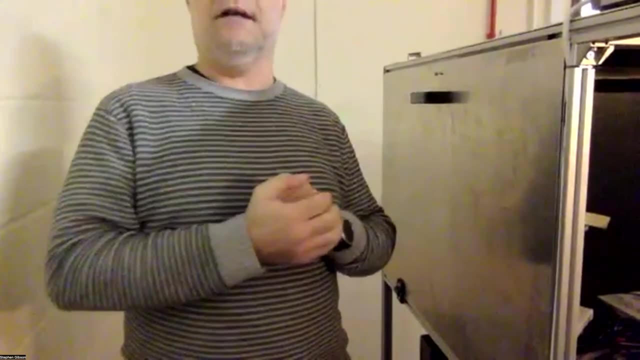 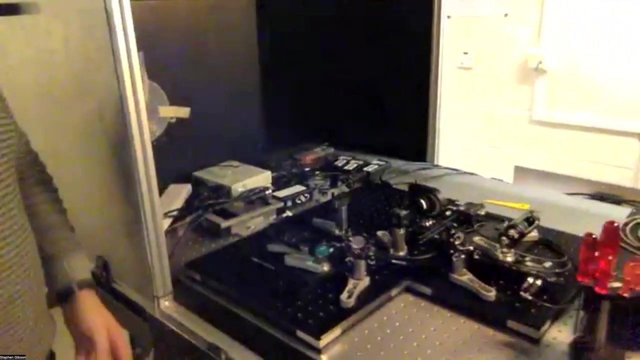 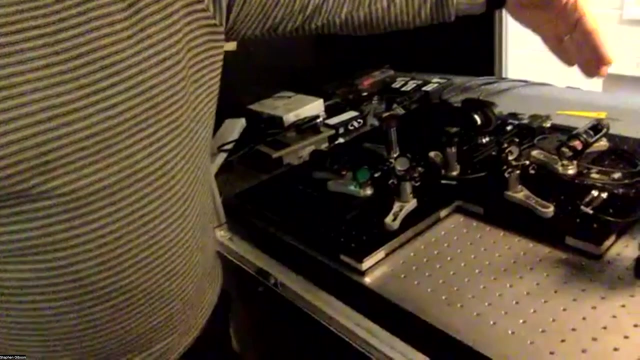 could select a beamlet made of only hydrogen ions, and this is then uh, for the downstream, we could measure this, the size and the divergence of this uh beamlet, and then from that sort of reconstruct the, the property of the of the incoming beam, um, so to do that, we have, uh, we have um sort of a scanner. so basically, uh, a translation stage is. 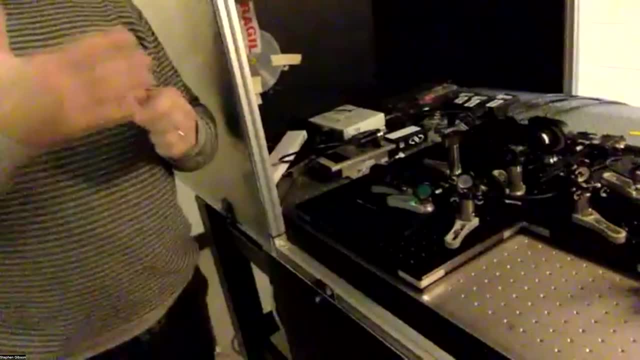 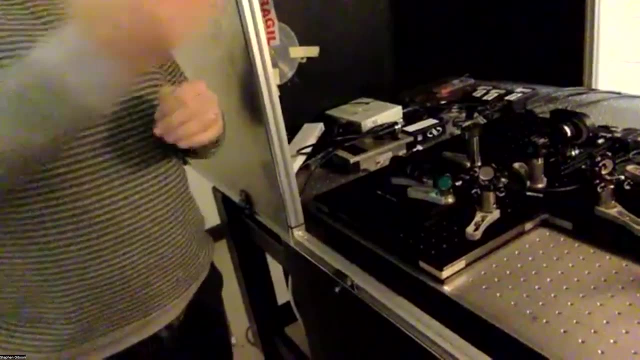 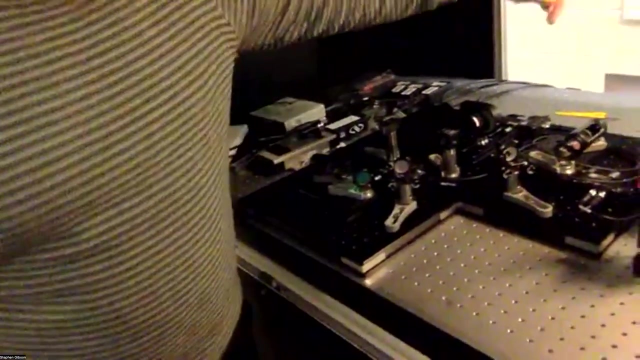 moving moves the, the laser beam across the, the, the accelerator, they accelerated the ions beam and then a different position. you have interactions and then, and then you can make your um, your reconstruction. so this, uh, this works with a laser that is sent into a fiber, an optical fiber, and 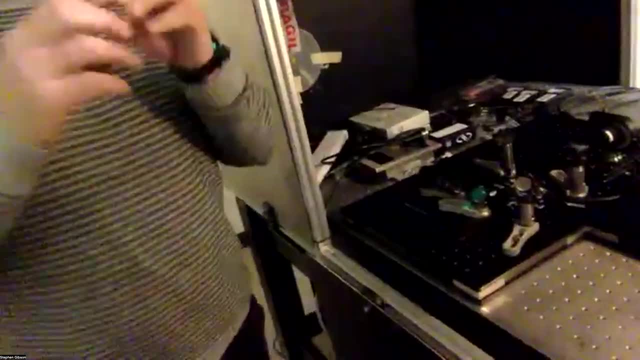 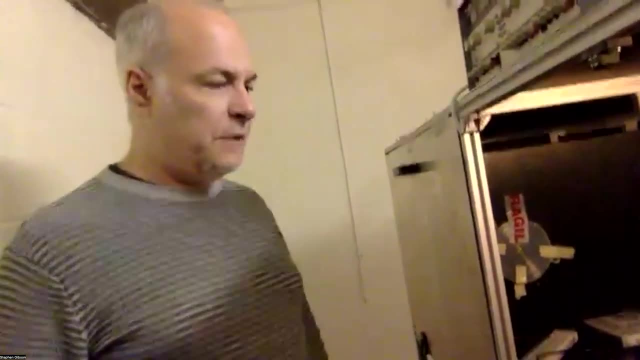 then the optical fiber end is attached to a translation stage and a lens that follows the laser, and then the translational stage is uh is is moved, and then, and then we, we could uh use it for that that purpose. um, so have we installed any other systems other than the one? 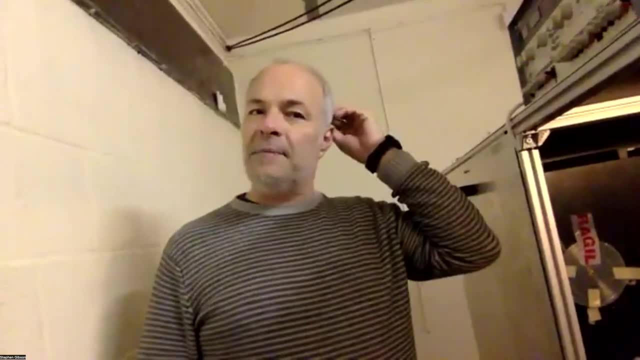 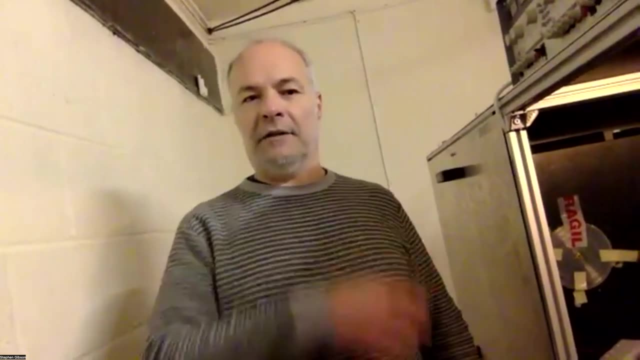 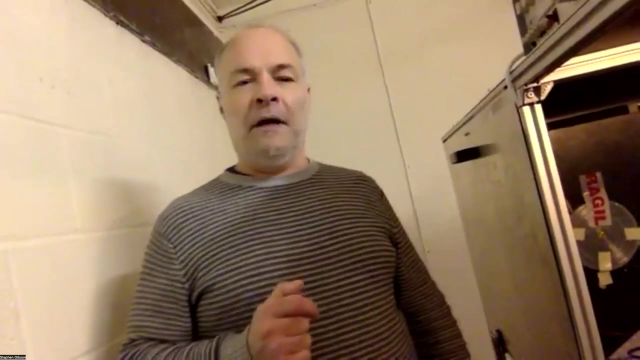 around. yeah, yeah, so this system has been, has been installed uh successfully at um, a Linux 4, which is, uh, again, it's an H minus accelerator, that is um, it's, it's used, uh, it's used uh for the for the LH and LHC and um, and 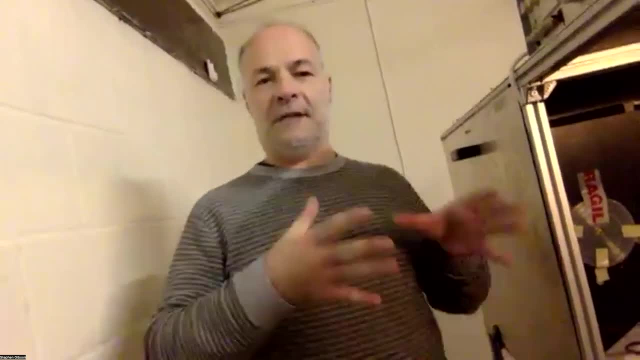 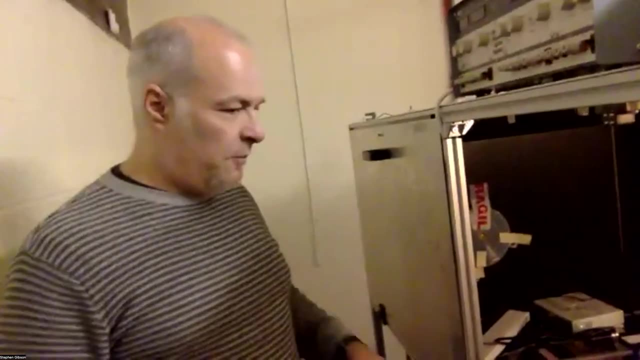 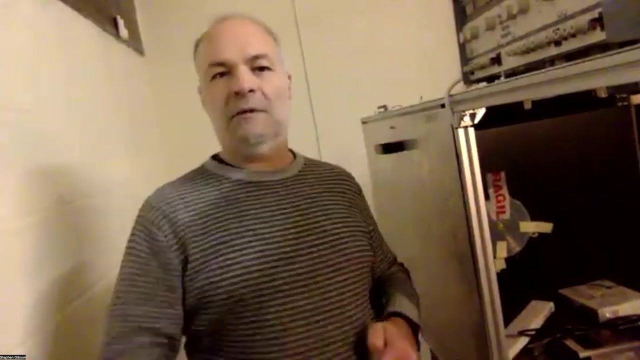 uh was uh. so we basically built one of these systems and then use it at the different locations within this accelerator to measure the beam as it was developed, as it was developed and it was uh, it was quite accessible- operation and other laser wires. so we did uh, but that was several years ago. 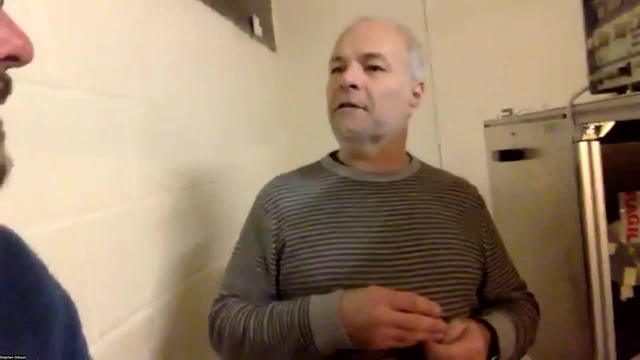 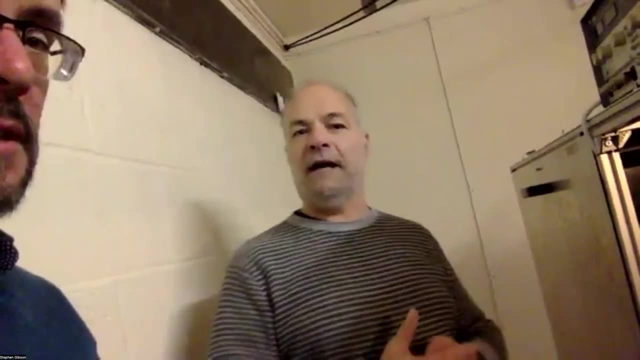 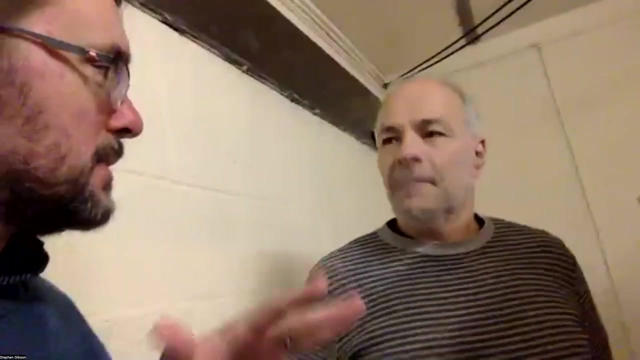 was for other accelerators, which were, uh, electron or positron accelerators. yeah, um, and, and the interaction was similar: laser with particle, but in another scale, which was more uh, yeah, yeah. so thank you. I'm aware time's short, but uh, I don't want to. yeah, but uh, yeah, thank you for. 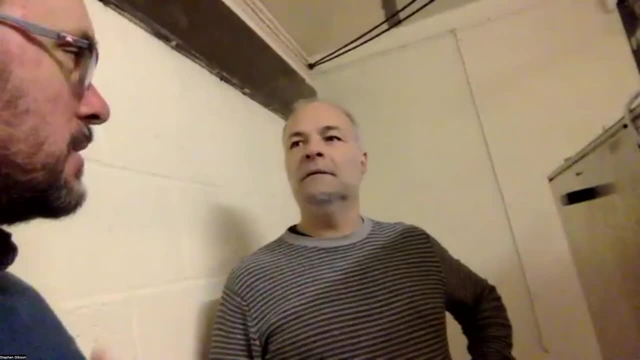 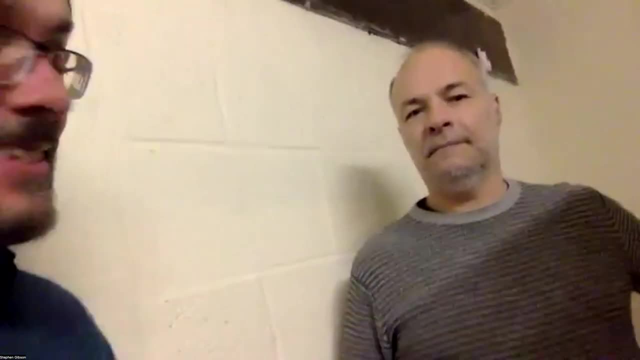 sharing us around. yeah, I mean. so this is the laser wire effects, but there's been a similar one at CERN LINAK 4 um, and then there's some over in PETRA 3 in DAISY and others out in Japan um at KK. so we